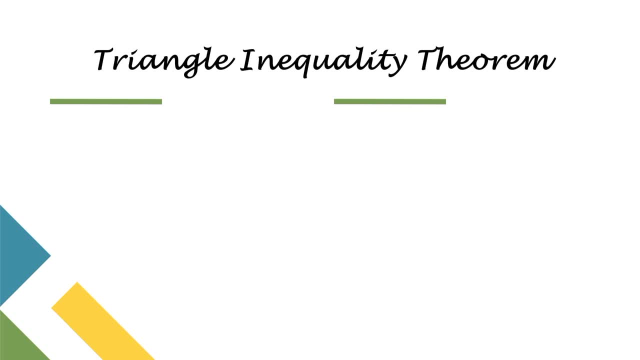 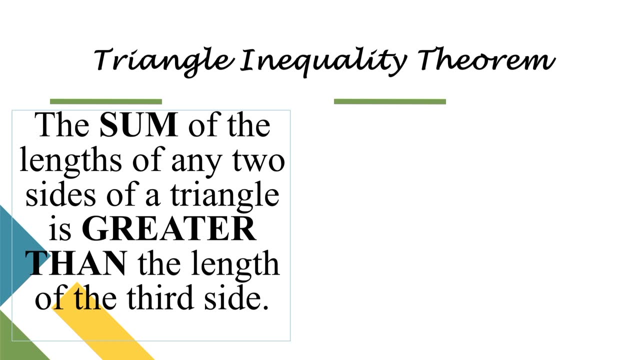 Okay, so when we are talking about triangle inequality theorem, the concept of this theorem is The sum of the lengths of any two sides of a triangle is greater than the length of the third side. So it means if we have three sides. so take note, or you need to recall your knowledge about the parts of a triangle. 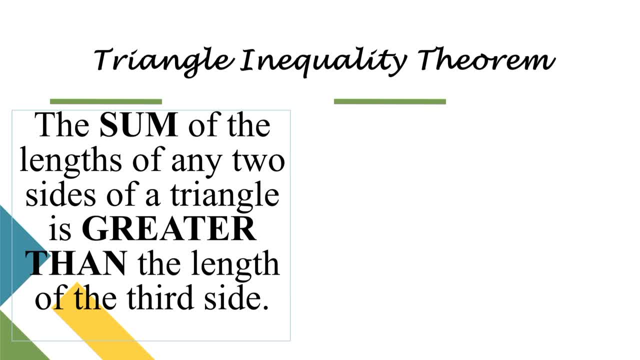 So when we are talking about triangle, it has three sides. Okay. so when we are talking about triangle, inequality theorem class, the concept of this one is: It says, It says, It says that the sum of the lengths of any two sides of a triangle is greater than the length of the third side. 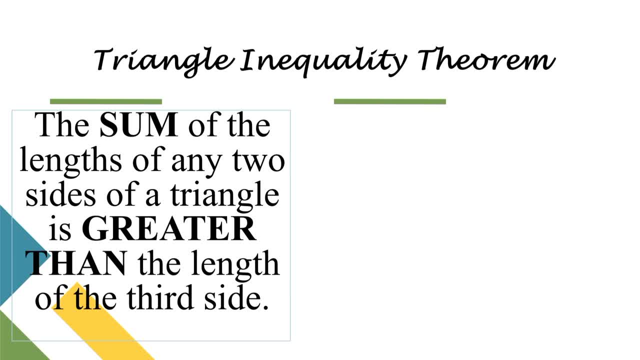 So if we add the two sides, the sum of the two sides should be greater than the length of the third side. So therefore we can say that A plus B is greater than C. A plus C is greater than B And the last one we have here, B plus C, is greater than A. 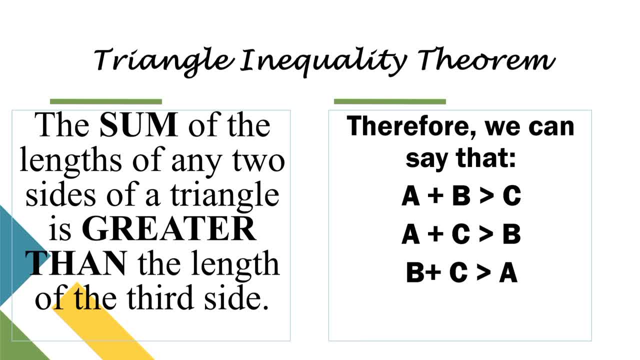 Okay, so is it clear. Okay, very good. So it means We will follow these statements to check if our solution is correct or our answer is correct, So you will be able to understand this one later on. Okay, so is it clear. 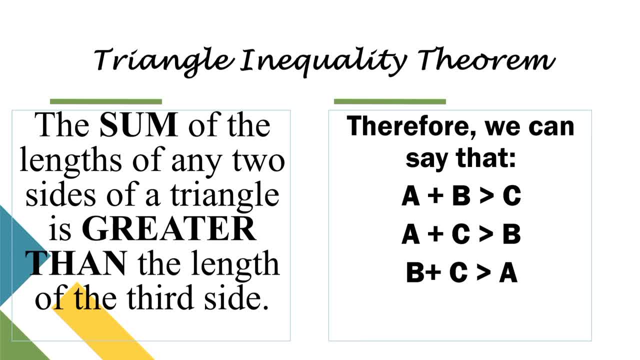 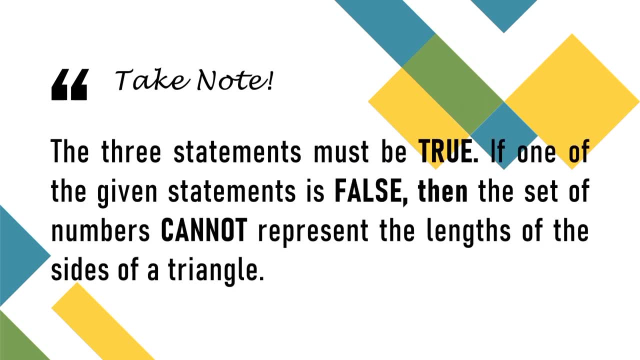 Okay, very good. So again, we will use these three statements in order to prove our answer is correct. Okay, so is it clear? Okay, very good. Okay, so you need to take note, class, that the three statements must be true. 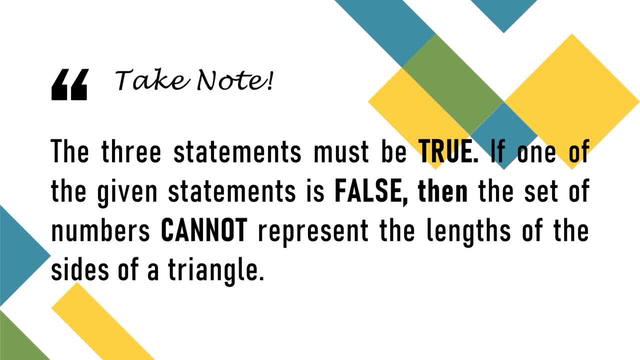 Okay, the A plus B is greater than C, A plus C is greater than B, And the last one, B plus C, is greater than A. So the three statements must be true. Okay, if one of the given statements is false, then the set of numbers cannot represent the lengths of the sides of a triangle. 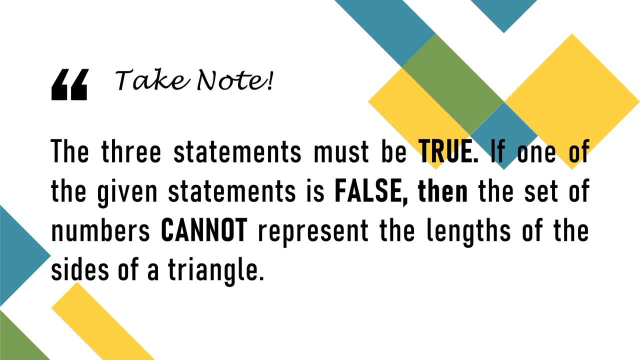 Okay, so if one of them is false, it means The set of the given numbers cannot represent the lengths of the sides of a triangle. Okay, so, even if the two statements are true, but one of them is false, therefore, the given set of numbers cannot represent the lengths of the sides of a triangle. 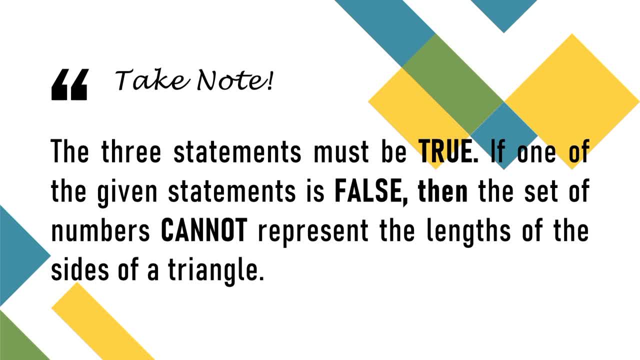 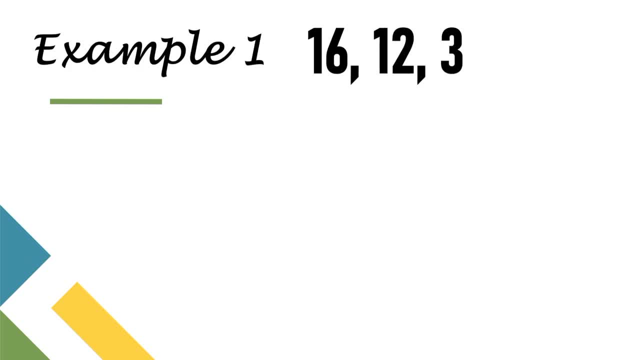 So the three statements must be true. Okay, so is it clear? Okay, very good. Okay, so we have here our example number one. For example, you are given this as Set of numbers. we have here 16,, 12, and 3.. 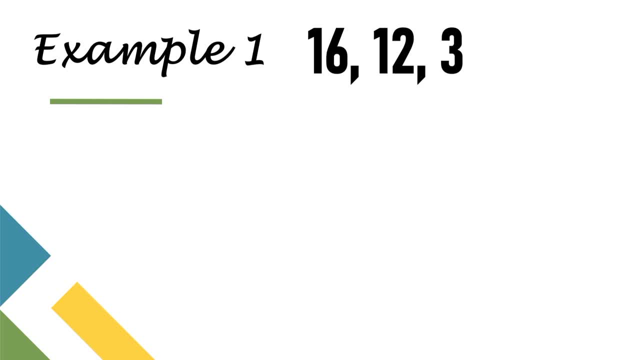 So let's check if these three numbers can represent the lengths of the sides of a triangle. So by using those three statements earlier. Okay, so let's assume that A is equal to 16,, B is equal to 12, and C is equal to 3.. 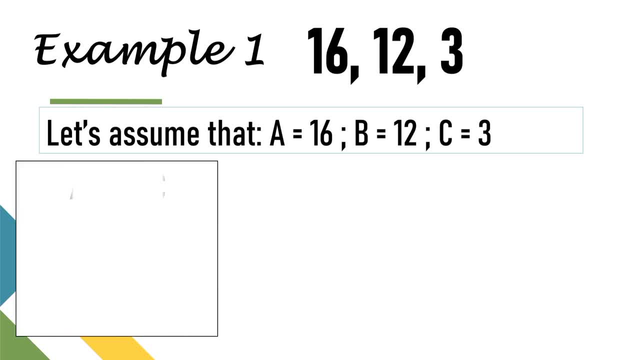 Okay, so let's start with the first statement. Okay, so we have here: A plus B is greater than C, So all we need to do is to substitute. So the value of our A is 16, and the value of our B is 12.. 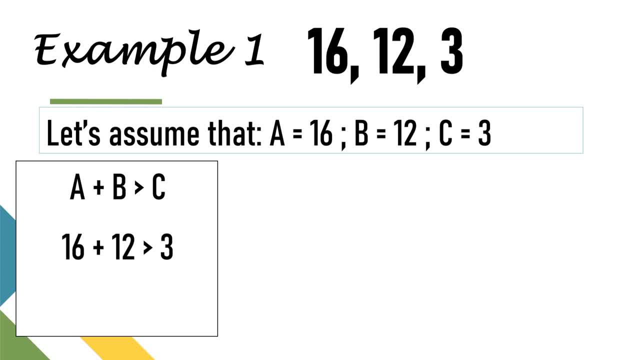 So 16 plus 12 is greater than the value of our C is 3.. So 16 plus 12, we have here 28.. So 28 is greater than 3, therefore our first statement is true. Okay, so again, let's check first the three statements before concluding. 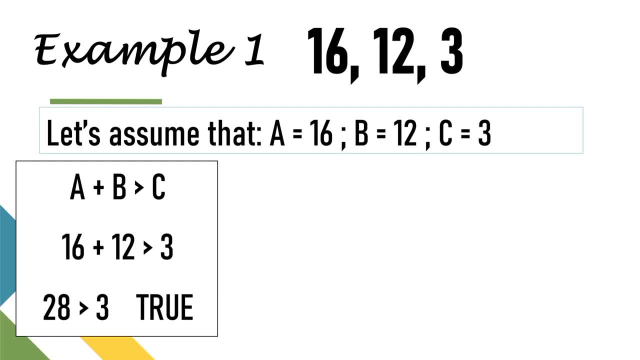 Okay, so we are done with our first statement and it is true. So let's check the second statement. So the second statement is: we have here A plus C. So the second statement is: we have here: A plus C is greater than B. 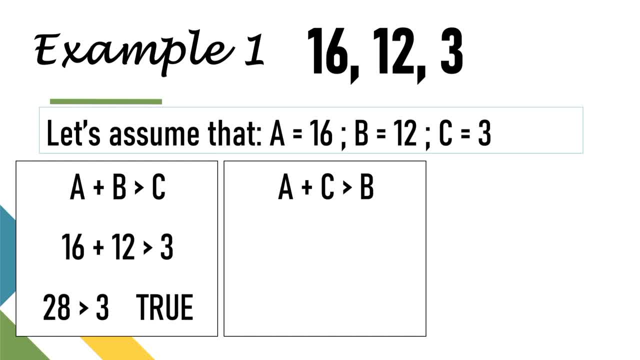 So let's substitute again. So the value of our A is 16, and the value of our C is 3.. So 16 plus 3 is greater than the value of our B is 12.. So 16 plus 3, we have here 19- is greater than 12.. 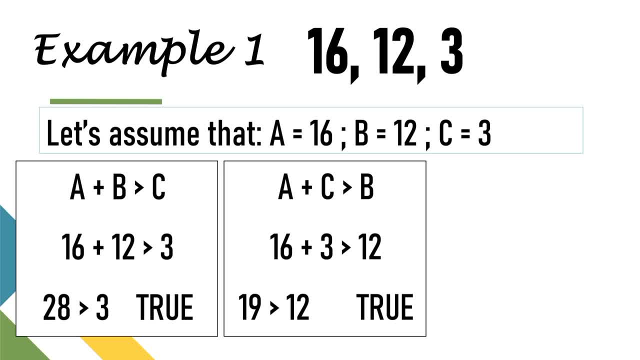 So 19 is greater than 12, therefore, our second statement is true. Okay, so we are done with our first and second statements, and they are true. So let's check our last statement, or the third statement: B plus C is greater than A. 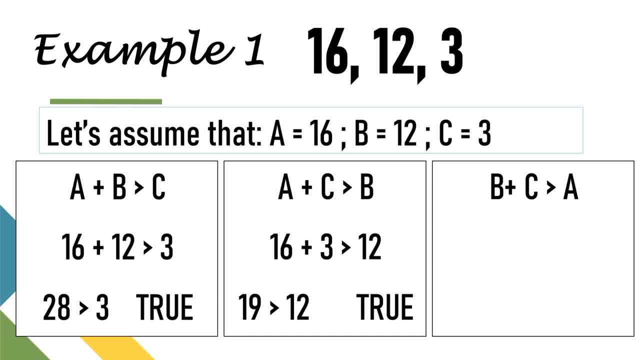 Again, all we need to do is the substitute. So the value of our B is equal to 12, plus the value of our C is equal to 3.. So we have here: 12 plus 3 is greater than the value of our A is 16.. 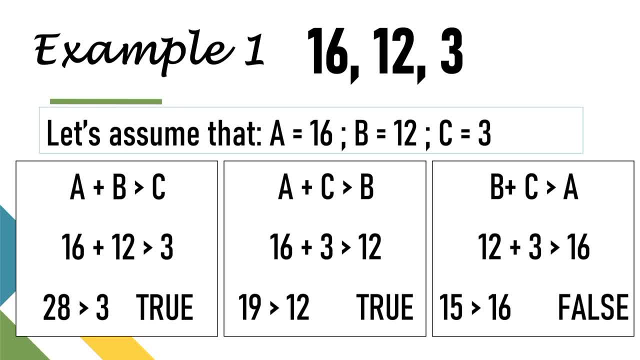 So 12 plus 3, we have here: 15 is greater than 16.. So is it true? No, Okay, why no? It's because 15 is not greater than 16.. Instead, 15 is less than 16.. 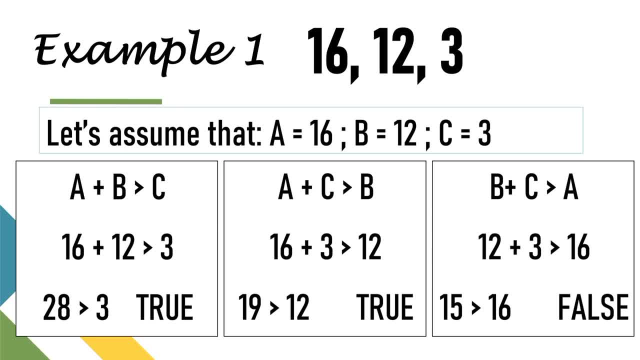 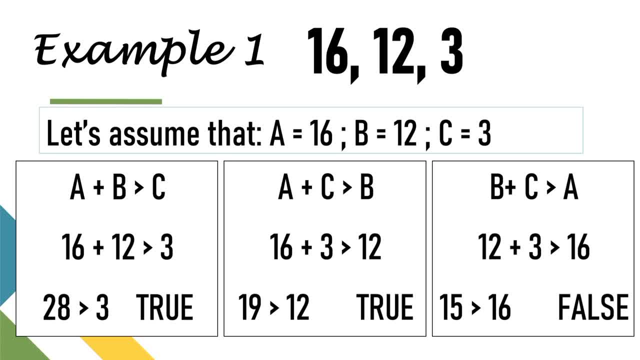 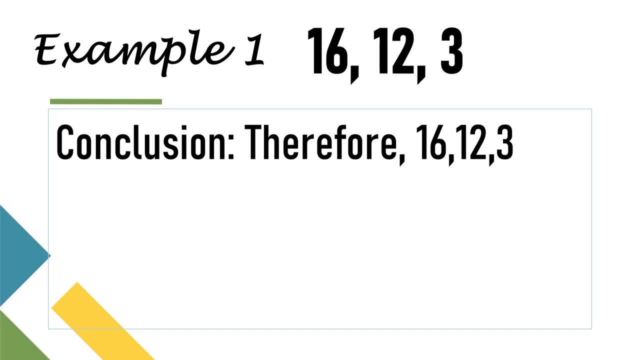 but there's one that is false. therefore, we can conclude that the given set of numbers cannot represent the length of the sides of A triangle. So let's proceed now to our conclusion. Okay, so we have here our conclusion. Therefore, 16,, 12, and 3 cannot represent the length of the sides of A. 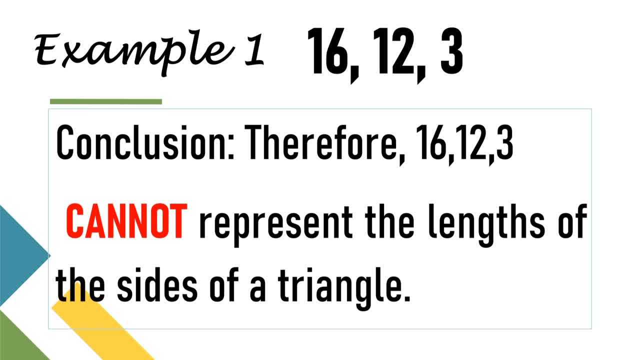 Okay, very good. So again, if ever the three statements are true, therefore, the given set of numbers can't represent the length of the sides of A triangle. So, based from our example, based from the given set of numbers, the given set of numbers, one statement is false. 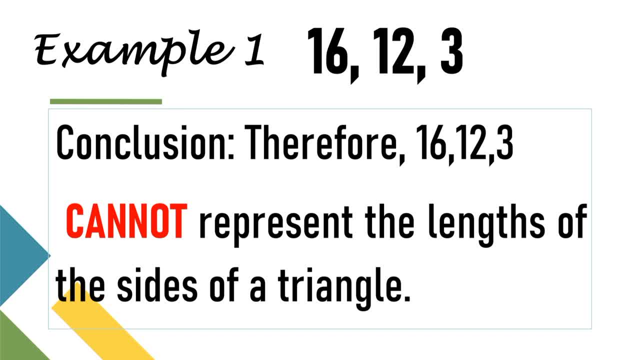 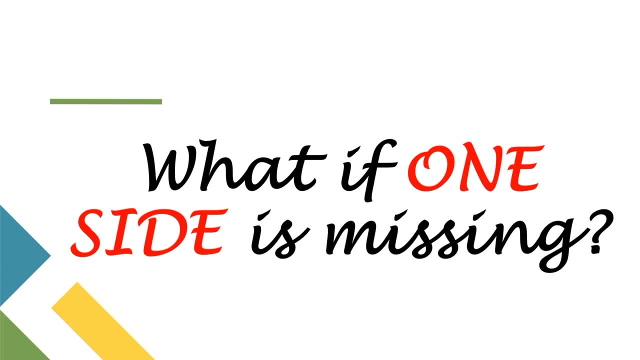 So therefore, the given set of numbers 16,, 12, and 3 cannot represent the length of the sides of A. Okay, try again. Okay, so did you understand? Okay, very good, What if one side is missing? 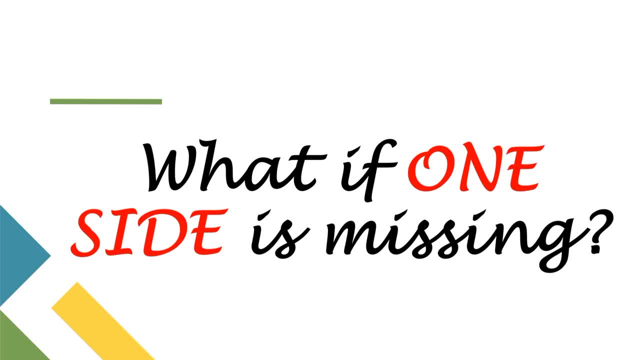 So, for example, you are given two sides only, or the measurement of the two sides only, and the one side is missing. So what are you going to do now? Okay, so let's proceed to the next slide, in order for us to know and understand. 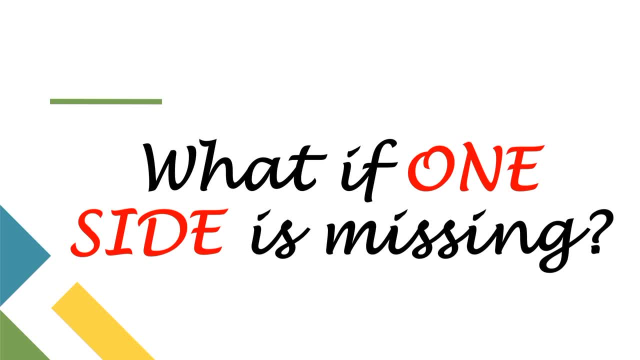 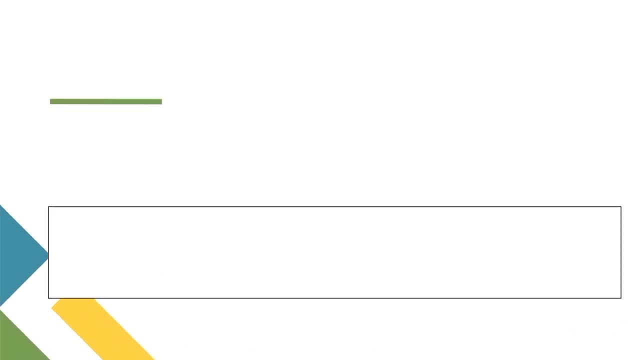 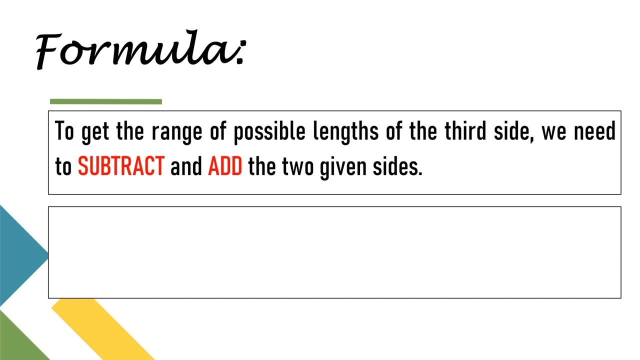 and how to solve if one side is missing. Okay, so did you understand? Okay, very good. Okay, so we have here our formula. okay, so this is what you will remember. okay, So to get the range of possible lengths of the third side. 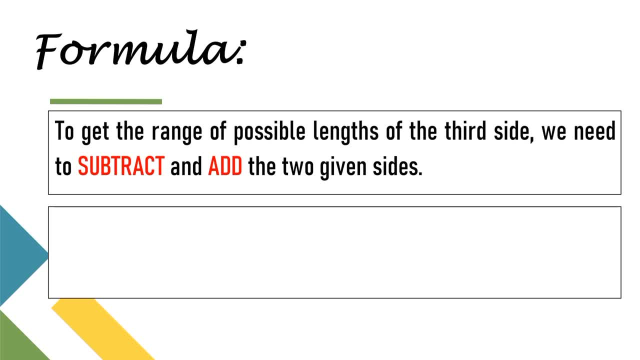 we need to subtract and add the two given sides. So therefore, class, we can say that a result of subtraction, or we can say that X is greater than the result of subtraction and less than with result of addition. Okay, teacher Kim, why are we looking for a range of possible lengths? 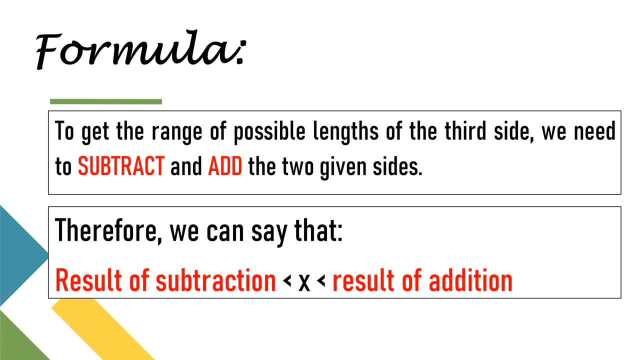 on our third side. Okay, it's because class we don't have an exact length of the third side, since our third side is missing. So therefore, we will find the range of possible lengths. Okay, So we are not looking for a single number. 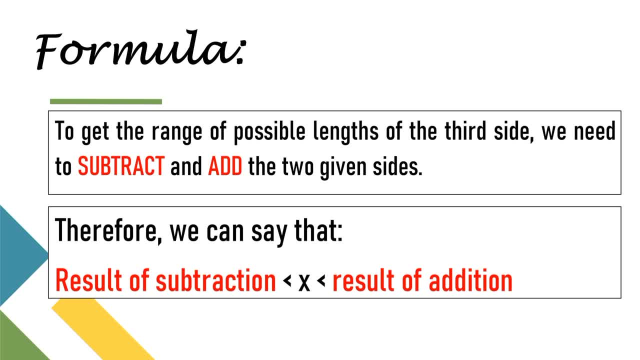 Okay, The range of possible lengths, lengths of the third side, so you will be able to understand it one later on. so again, you need to keep in mind that this statement X is greater than the result of the subtraction, but less than with the result of addition. dahil gagamitin natin yan. 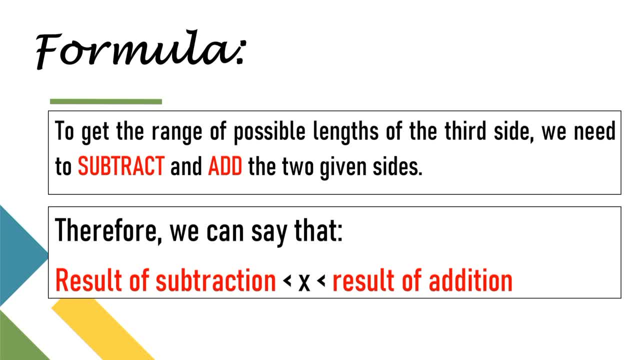 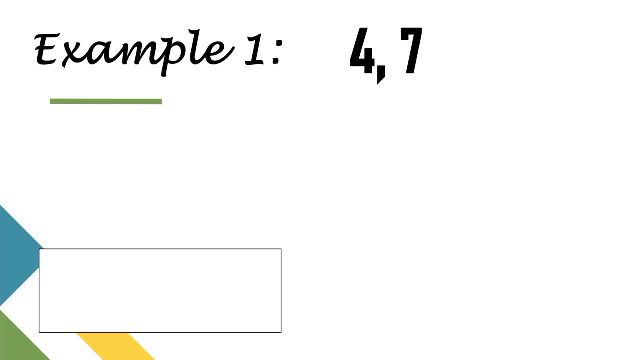 later on. so all we need to do is to subtract and add the two given sides so you will be able to understand it one later on. so is it clear? okay, very good, let's start with our example number one. so, for example, you are only given four. 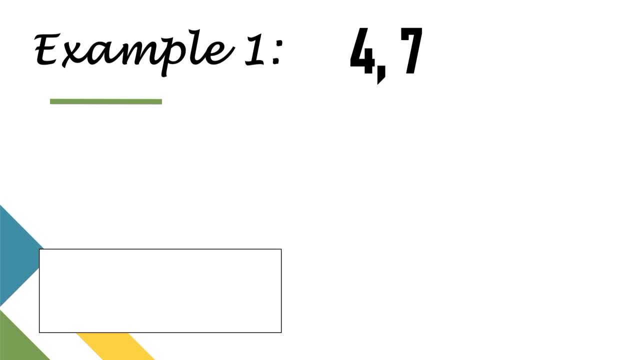 and seven. so, based from your observation, meron lang tayong two sides so missing, see one side. okay, the measurement of the other side or the third side. so again, take note that the solution is to get the range of possible lengths of the third side. we need to. 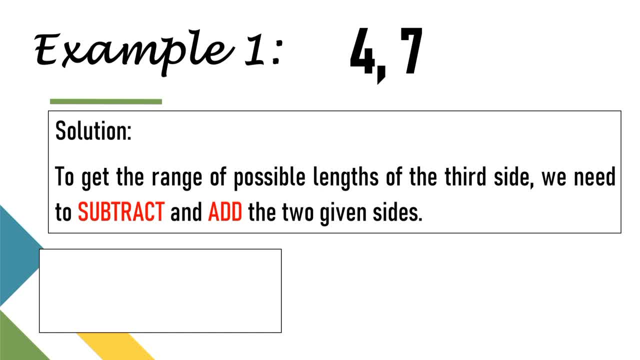 subtract and add the two given sides. okay. so let's start with subtraction. so we have here: seven minus four is equal to three. okay, teacher Kim, ah di ba pwedeng four minus seven. okay, take note class na we don't have a measurement na negative, so therefore dapat mauna yung pinakamalaking number. 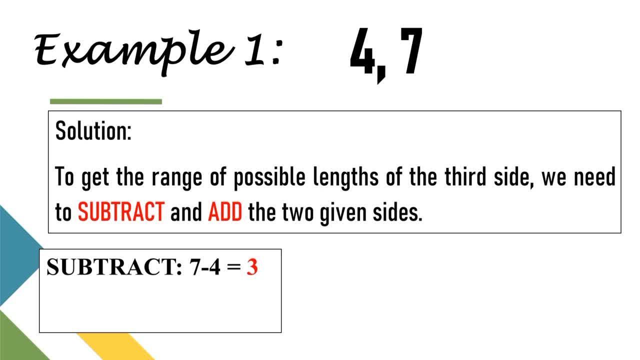 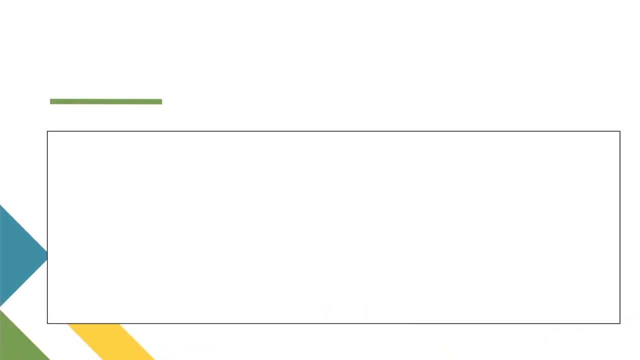 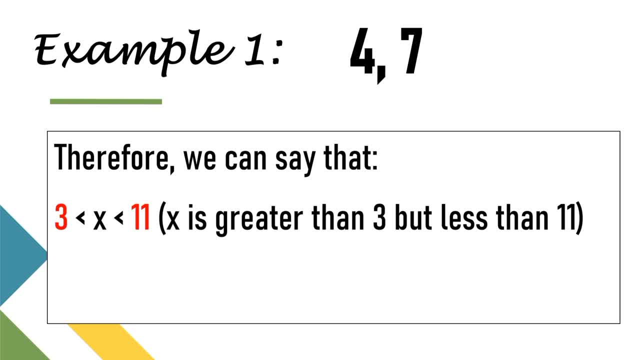 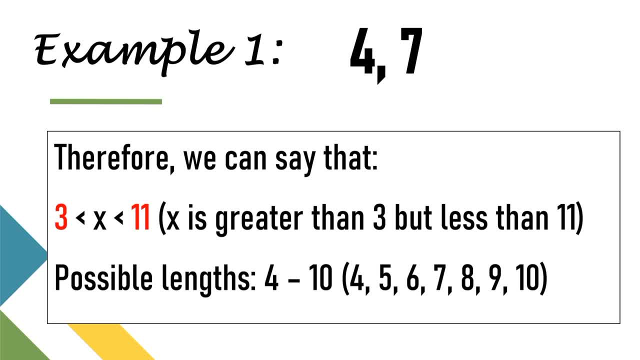 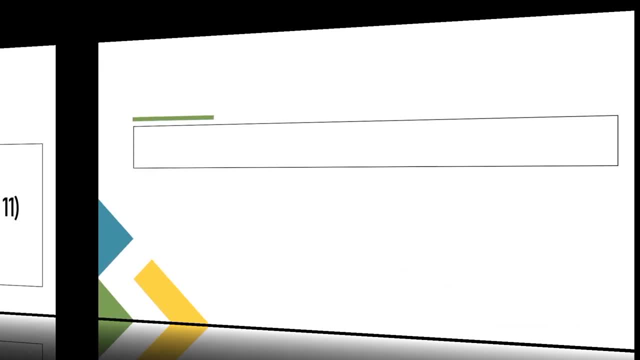 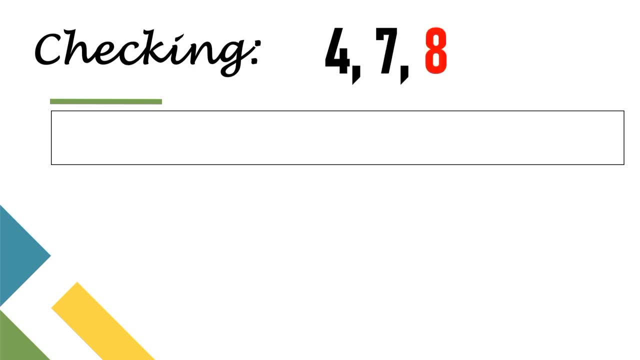 Okay, very good. Okay, so let's have now our checking. So we have here 4,, 7, and 8.. So, based from your observation, class 8 is in red, so you won't get confused. Okay, so we have our possible length, so 4 to 10.. 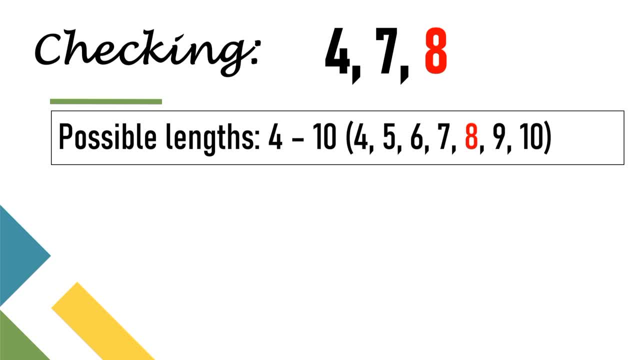 So we have here 4,, 5,, 6,, 7,, 8,, 9,, 10.. Okay, so, so as not to consume time, so we will only get one number from possible lengths, or the range of possible lengths of the third side. 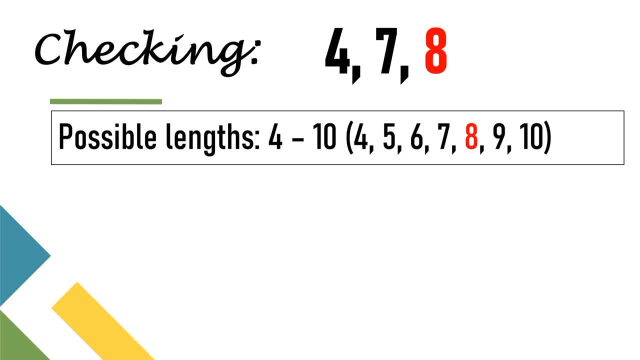 So yung napili ko is si 8.. But you can choose either 4,, 5,, 6,, 7,, 8,, 9, or 10. It's up to you. As long as pwede lang isa yung itch check ninyo. 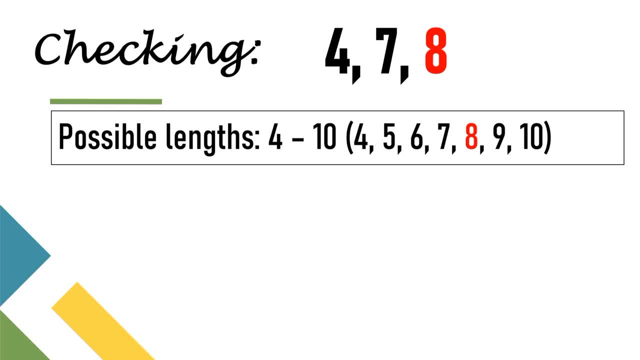 So in my case, I will use 8 to check whether the given set of numbers- the 4,, 7, and 8, are or can represent the lengths of the third side. Okay, so we have here our first statement, or first. 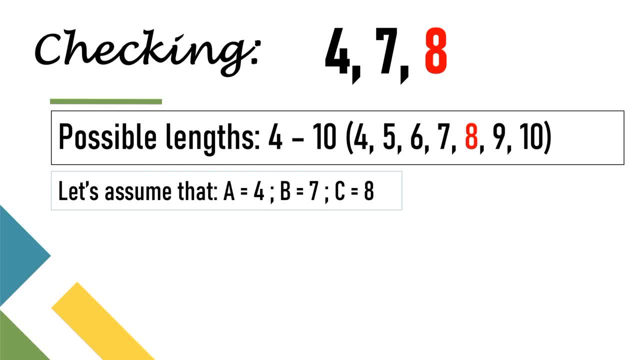 let's assume that A is equal to 4,, B is equal to 7, and C is equal to 8.. Okay, so let's start with our first statement. So we have here our first statement: A plus B is greater than C. 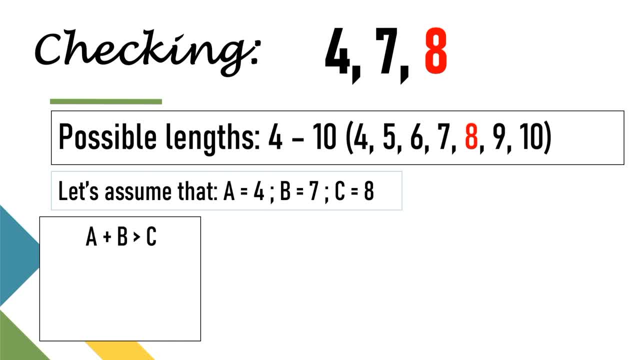 So again, all we need to do is to substitute. So the value of our A is 4 and the value of our B is equal to 7.. So we have here: 4 plus 7 is greater than the value of our C is equal to 8.. 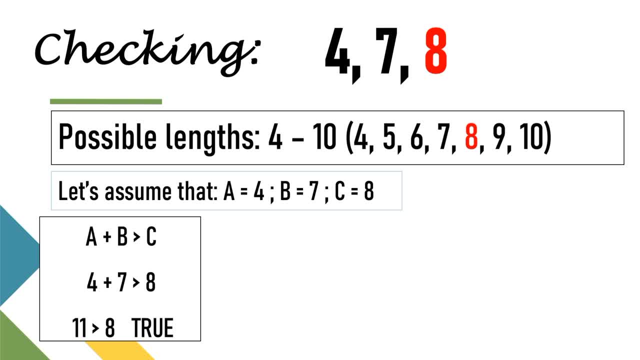 So we have here 4 plus 7, we have here: 11 is greater than 8.. And our first statement is true. Okay, so ang ating first statement is true. Let's check the second statement. So we have here our second statement: A plus C is greater than B. 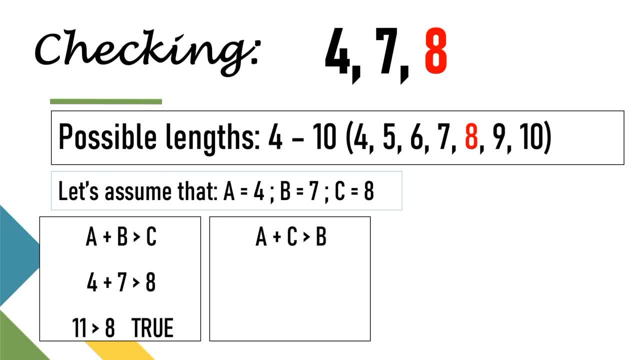 So again, let's substitute only. So the value of our A is equal to 4 and the value of our C is equal to 8.. So we have here: 4 plus 8 is greater than 7.. 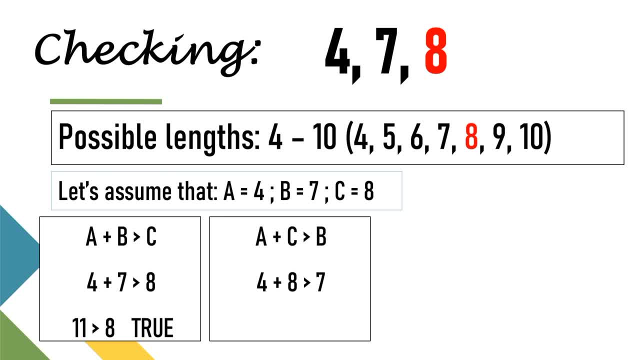 Okay, so the value of our B is equal to 7.. So 4 plus 8, we have here 12. So 12 is greater than 7. And our second statement is true. So, as you observe, yung first and second statements are true. 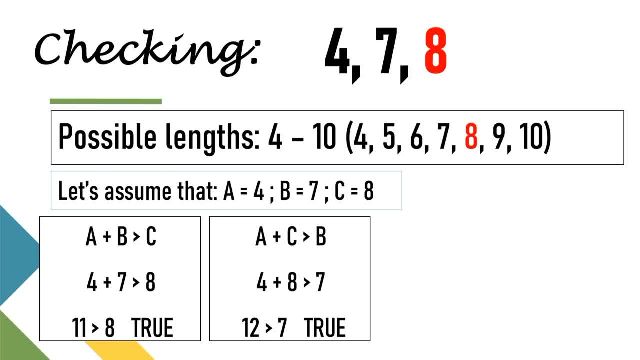 So let's check the third statement. if true, ba siya. Okay. so we have here our third statement. B plus C is greater than 8.. So the value of our B is equal to 7 and the value of our C is equal to 8.. 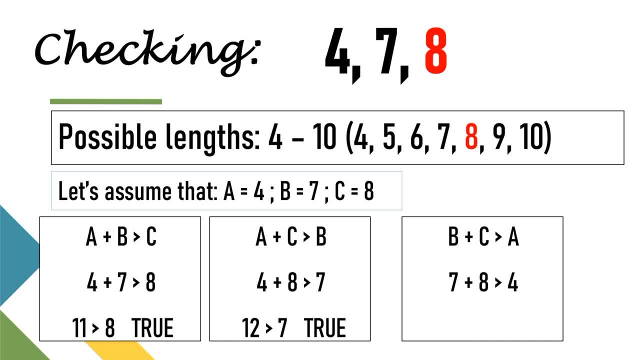 So we have here: 7 plus 8 is greater than 8.. So the value of our A is equal to 4.. So 7 plus 8, we have here 15 is greater than 4.. And our third statement is true. 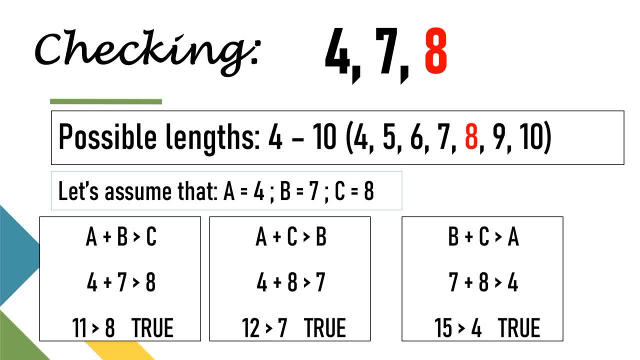 So therefore, class yung possible lengths natin are true. Okay, So is it clear? Okay, very good. So again, in checking, all you need to do is to get only one number only. Okay, So, para hindi consuming ng time, 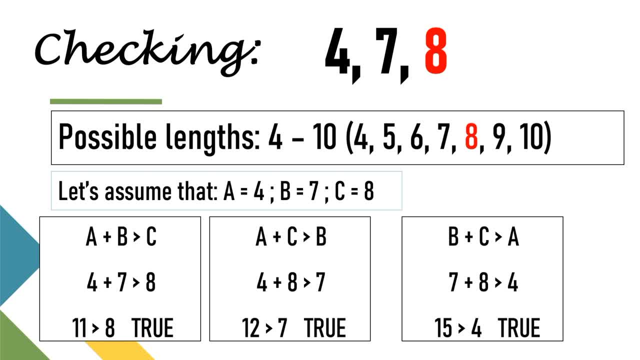 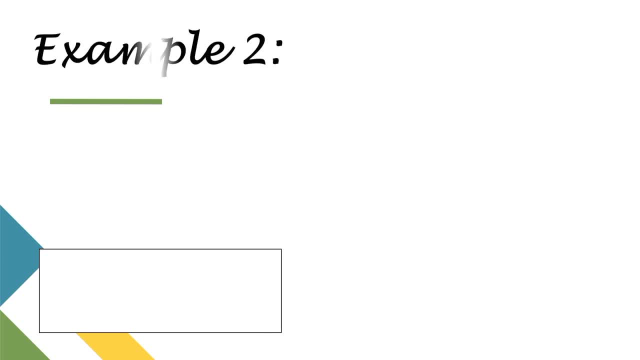 Okay, So is it clear. Okay, Very good. Okay, so we are done with our example number 1, our first example. So now let's proceed to our example number 2.. We are given only 3 and 9.. 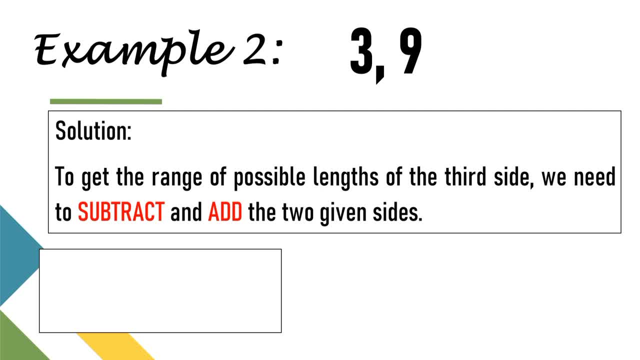 Okay, So what are we going to do? Our solution: to get the range of possible lengths of third side, we need to subtract and add the two given sides. So we have here, let's do first the subtraction. So we have here, subtract 9 by 3.. 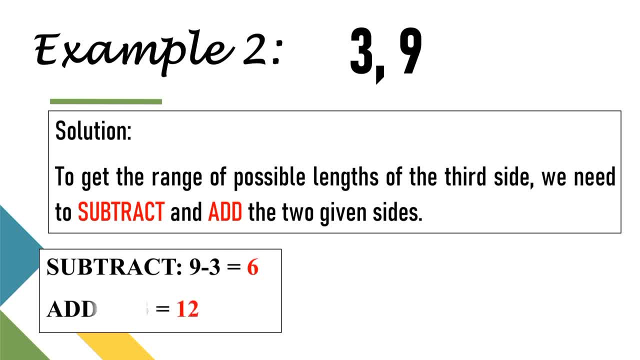 So 9 minus 3, we have here 6.. And addition, we have here 9 plus 3.. We have here 12.. So again, the result of our subtraction is equal to 6, or the difference is 6 and the. 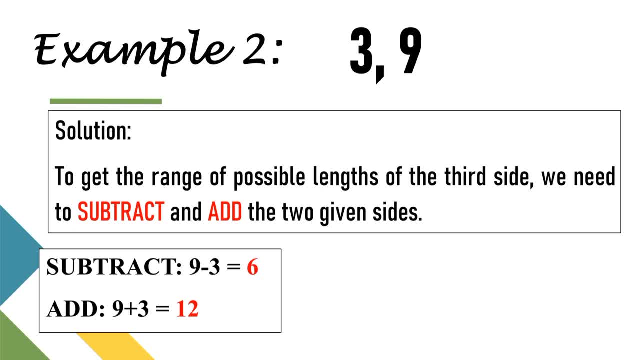 sum is 12.. So again, the result of our subtraction, we have here 6, and the result of our addition, we have here 12.. So don't forget that one. it's because we will use that one on the next slide. 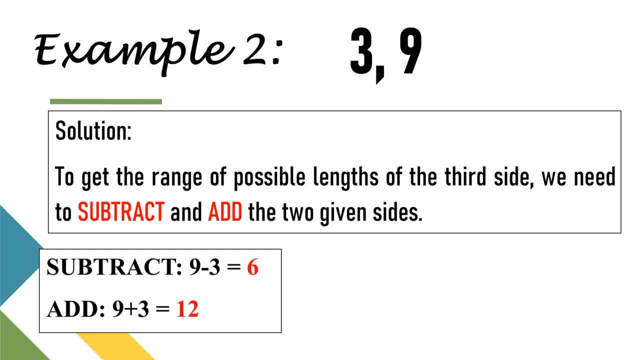 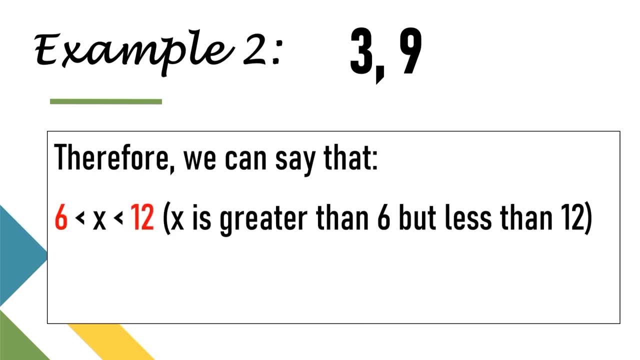 Okay, So is it clear. Okay, Very good. Okay, So we have here, Therefore, we can say that the terms that we've deducted here are none. so we have here. therefore, we can say that x is greater than 6 but less than 12. so again, the 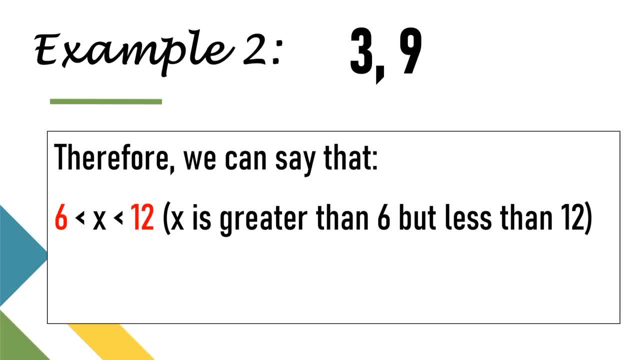 result of our subtraction is 6, uh, then use after 6. we will uh put greater than sign than x, then less than sign than 12, and it is read as x is greater than 6 but less than 12, so our possible length we have here x tau is greater than 6, so therefore 7. so what is a number that is greater? 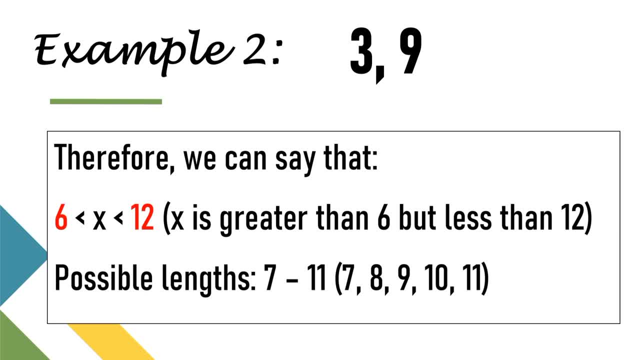 than 6. we have here 7, 2 less than 12, so we have here 11. so 7 to 11. we have here our possible lengths. we have here 7, 8, 9, 10 and 11. so these are the numbers that will be the possible lengths of. 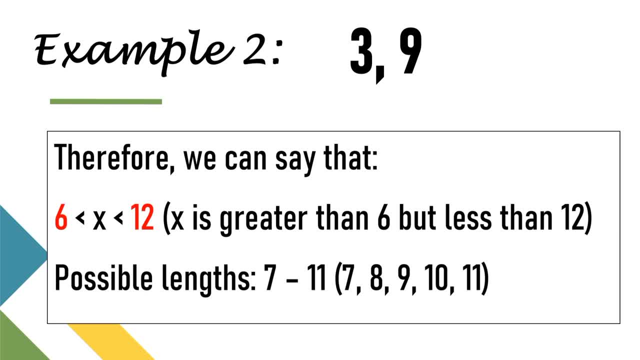 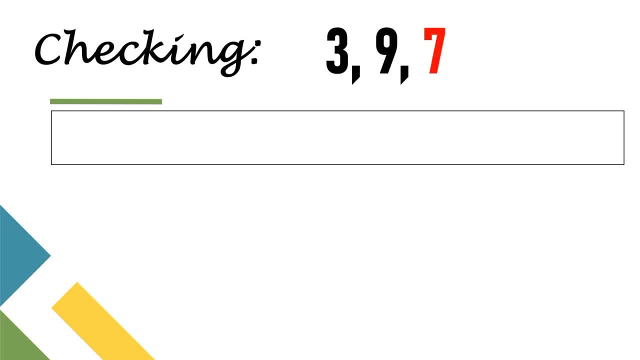 the third side. so let's check on the next slide. okay, so is it here? okay, very good, okay. so we have here our checking: 3, 9 and 7. so again, our possible lengths. we have here 7, 9, 10 and 11. so we have here our possible lengths. we have here 7, 9, 10 and 11. 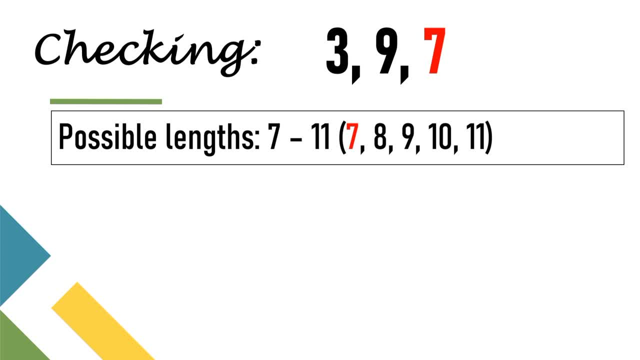 we have here 7 to 11. we have here 7, 8, 9, 10, 11.. in my case, i chose 7, okay, as the length of the third side. okay, so let's check. let's assume that a is equal to 3, b is equal to 9 and c is equal to 7, so 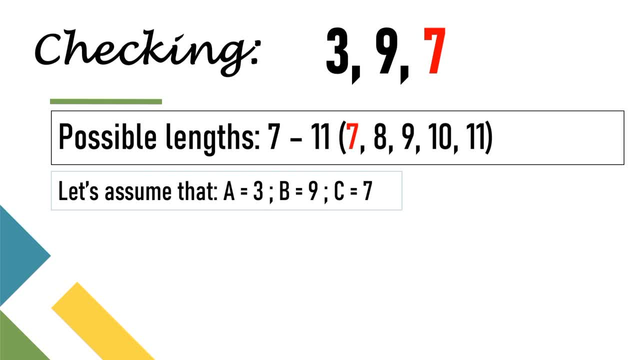 let's check this one using the three statements. so let's check first the three. uh, the first statement. so we have here: a plus b is greater than c, so all we need to do is the substitute. the value of our a is equal to 3, so we have here: a plus b is greater than c, so all we need to do is: 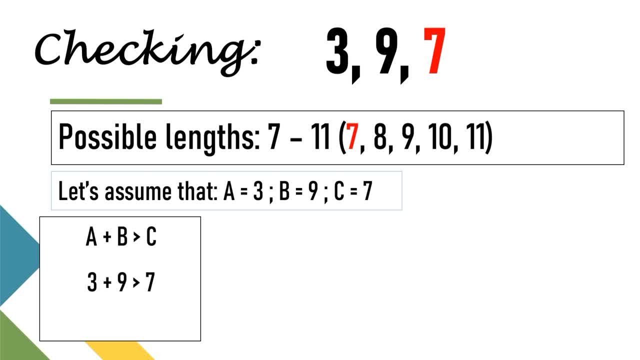 the substitute. the value of our a is equal to 3 and the value of our b is equal to 9. so we have here: and the value of our b is equal to 9. so we have here: 3 plus 9 is greater than the value of our c is. 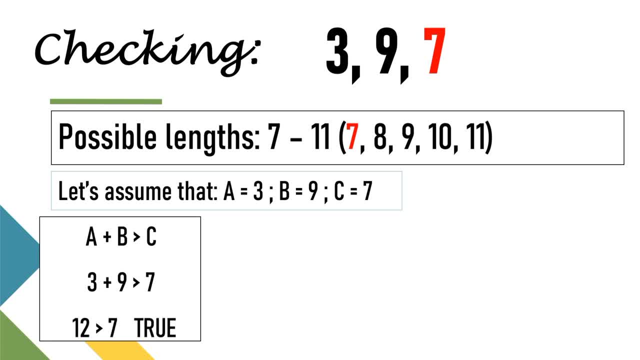 3 plus 9 is greater than the value of our c is 3 plus 9 is greater than the value of our c is 7. so 3 plus 9 we have here 12 is greater than 7. so 3 plus 9 we have here 12 is greater than. 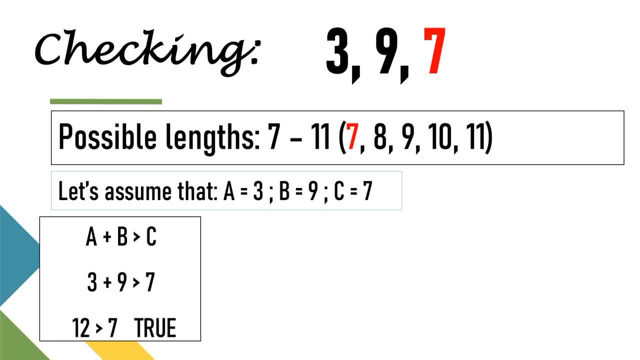 7, so 3 plus 9. we have here 12 is greater than 7, and our first statement is true. okay, so let's 7, and our first statement is true. okay, so let's 7 and our first statement is true. okay, so let's check the second statement. we have here a plus c. 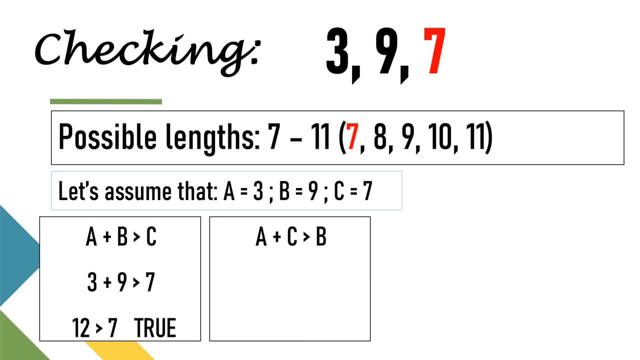 check the second statement we have here: a plus c. check the second statement we have here: a plus c is greater than b. okay, so all we need to do again is greater than b. okay, so all we need to do again is greater than b. okay, so all we need to do again is to substitute: the value of our a is equal to is to substitute. the value of our a is equal to is to substitute: the value of our a is equal to 3 and the value of our c is equal to 7, so we 3 and the value of our c is equal to 7, so we: 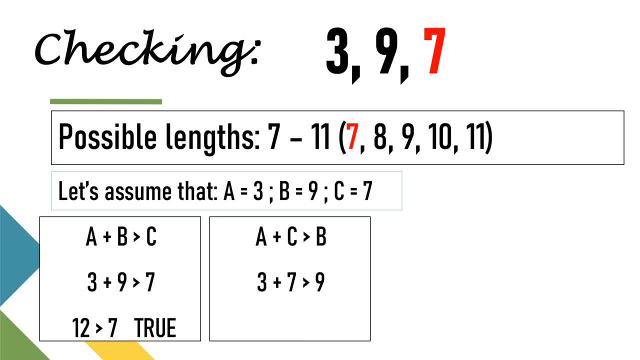 3 and the value of our c is equal to 7. so we have here: 3 plus 7 is greater than 9. so have here: 3 plus 7 is greater than 9. so have here: 3 plus 7 is greater than 9. so 3 plus 7- we have here 10- is greater than. 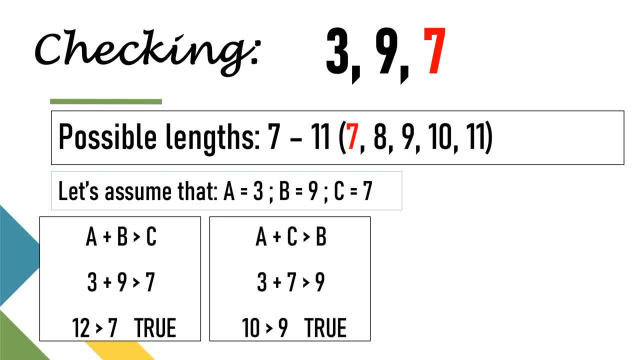 3 plus 7. we have here 10 is greater than 3 plus 7. we have here: 10 is greater than 9, then our second statement is true: okay, 9. then our second statement is true: okay, 9. then our second statement is true: okay, so proceed. dials the third statement. so. 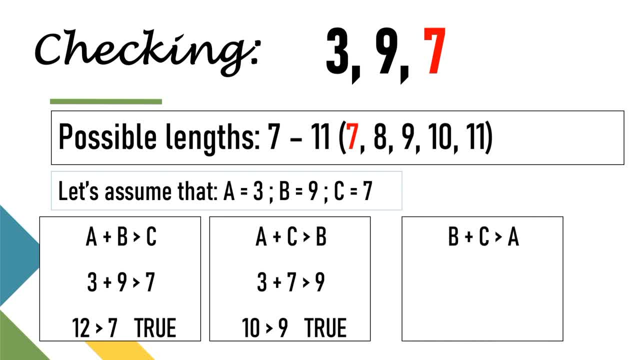 so proceed. dials the third statement. so so proceed. dials the third statement. so we have here our third statement, b plus. we have here our third statement, b plus. we have here our third statement: b plus c is greater than a the value of our b. c is greater than a the value of our b. 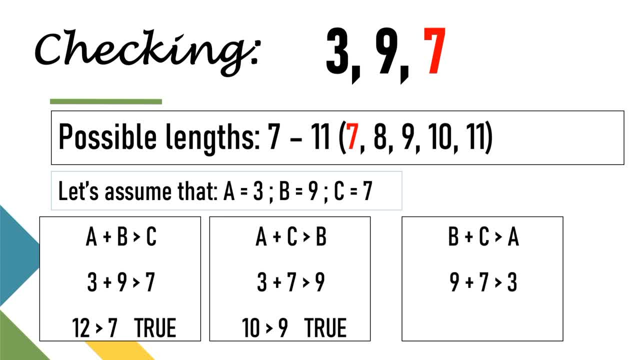 c is greater than a, the value of our b is equal to 9 and the value of our c? is is equal to 9 and the value of our c? is is equal to 9 and the value of our c is equal to 7 is greater than the value of. 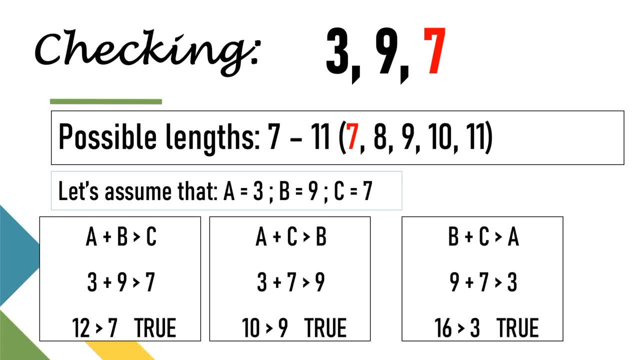 equal to 7 is greater than the value of equal to 7 is greater than the value of our. a is equal to 3, 9 plus 7. we have our a is equal to 3, 9 plus 7. we have our a is equal to 3, 9 plus 7. we have here 16 is greater than 3. therefore, our 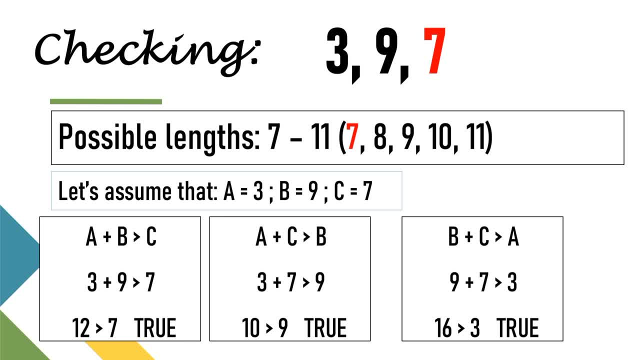 here 16 is greater than 3. therefore, our here 16 is greater than 3. therefore, our third statement is true. so, based from third statement is true. so, based from third statement is true. so, based from the given checking all of the three, the given checking, all of the three. 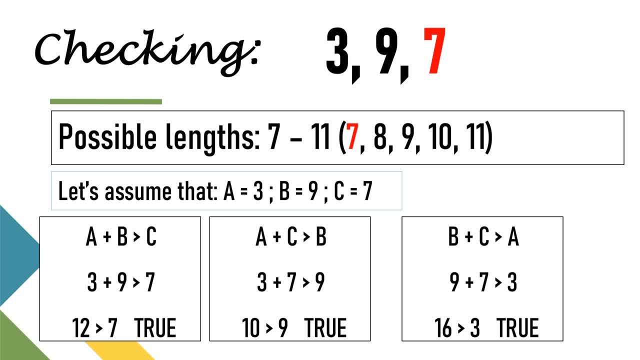 the given checking, all of the three statements are true. so therefore, uh, the statements are true. so therefore, uh, the statements are true. so therefore, uh, the possible lengths are two: okay, so you can. possible lengths are two: okay, so you can. possible lengths are two: okay, so you can check the other uh, numbers that will be. 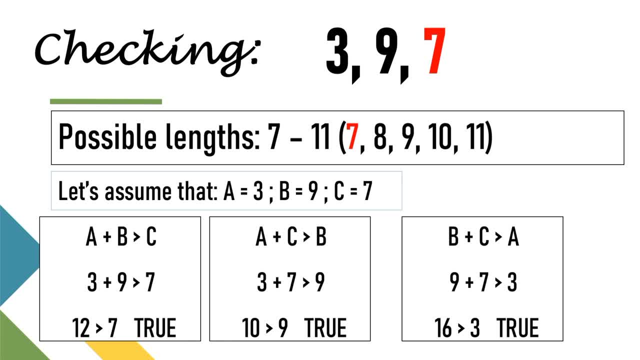 check the other uh numbers that will be. check the other uh numbers. that will be: uh, the possible lengths of the third side. uh, the possible lengths of the third side. uh, the possible lengths of the third side. we have here eight, nine, ten eleven. so we have here eight, nine, ten eleven, so 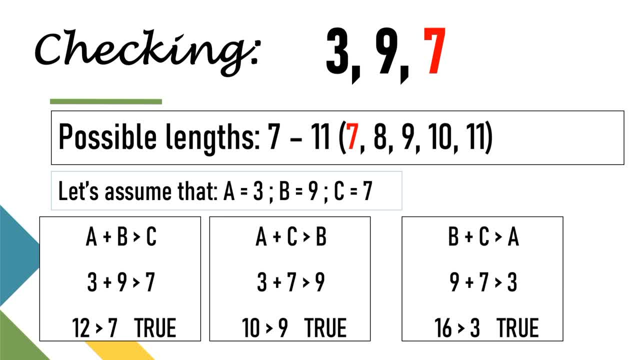 we have here eight, nine, ten, eleven, so you can check that one. so again, all you, you can check that one. so again all you, you can check that one. so again, all you need to do is to get one number based. need to do is to get one number based. 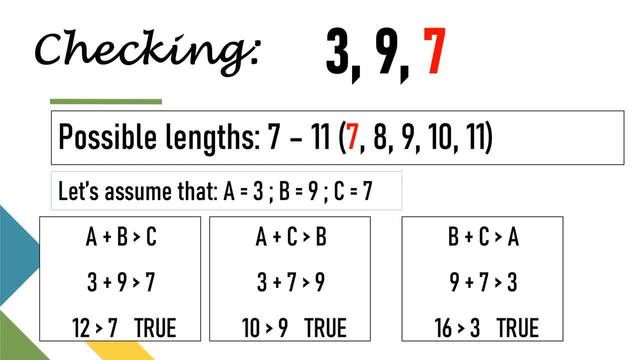 need to do is to get one number based from the given possible lengths. okay, so, from the given possible lengths. okay, so, from the given possible lengths. okay, so is it clear? is it clear? is it clear? okay, very good. okay, so we are done with our second. okay, so we are done with our second. 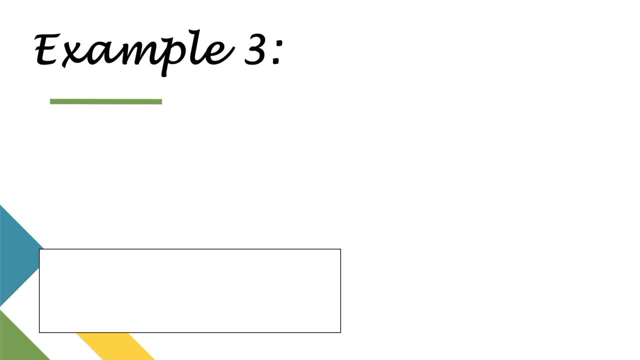 okay, so we are done with our second example. so now proceed to example number example. so now proceed to example number example. so now proceed to example number three. so we have here 20 and 13, so again three. so we have here 20 and 13, so again. 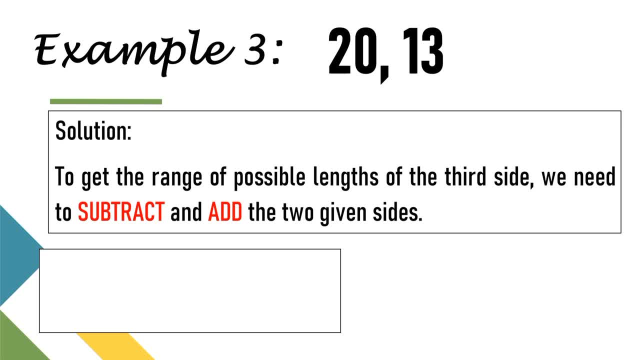 three. so we have here 20 and 13. so again, to get the range of possible lengths of, to get the range of possible lengths of, to get the range of possible lengths of the third side, we need to subtract and the third side we need to subtract and. 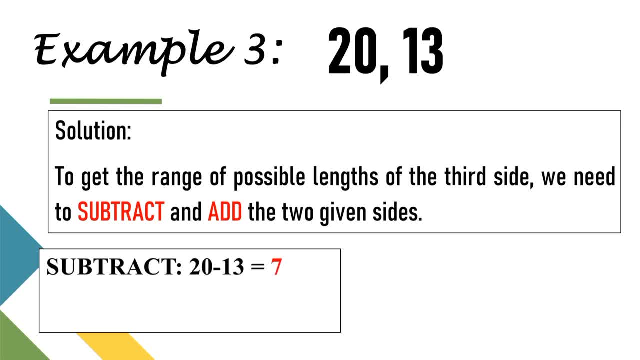 the third side, we need to subtract and add the two given sides. okay, so we have add the two given sides. okay, so we have add the two given sides. okay, so we have here subtract 20 by 13, so 20 minus 13. we here subtract 20 by 13, so 20 minus 13. we. 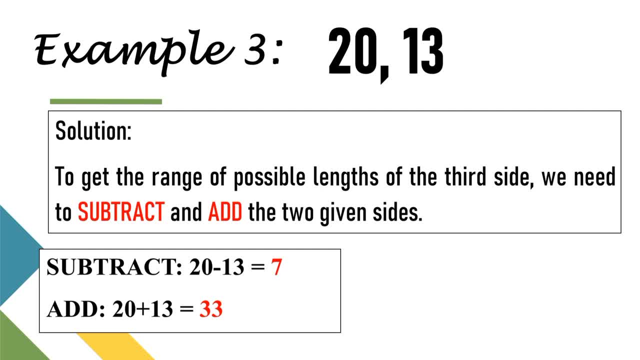 here: subtract 20 by 13. so 20 minus 13, we have here seven and we need to add 20. have here seven and we need to add 20. have here seven and we need to add 20 plus 13. we have here 33. so the result of: 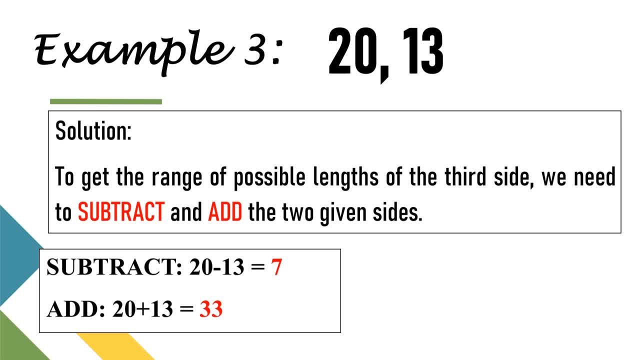 plus 13, we have here 33. so the result of plus 13, we have here 33. so the result of our subtraction is equal to 7 and the our subtraction is equal to 7 and the our subtraction is equal to 7 and the result of our addition is 33 or the. 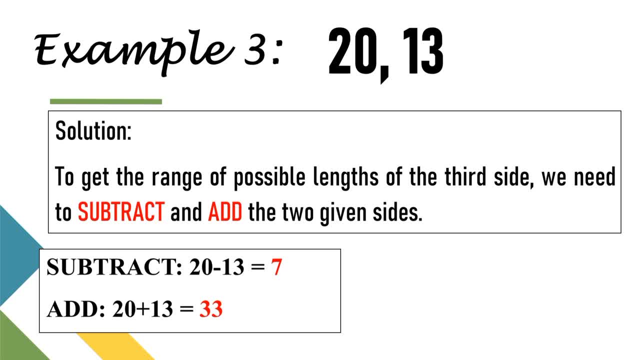 result of our addition is 33. or the result of our addition is 33, or the difference is 7 and the sum is 33, so difference is 7 and the sum is 33, so difference is 7 and the sum is 33. so don't forget that one. okay, so is it. 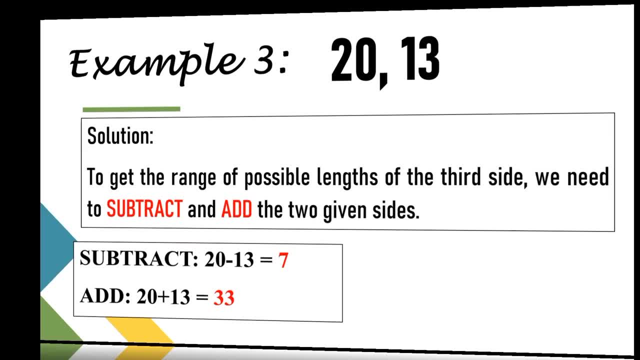 don't forget that one. okay, so is it? don't forget that one. okay, so is it here. okay, very good, okay, so we have here. therefore we can. okay, so we have here, therefore we can. okay, so we have here. therefore, we can say that x is greater than 7, but less. 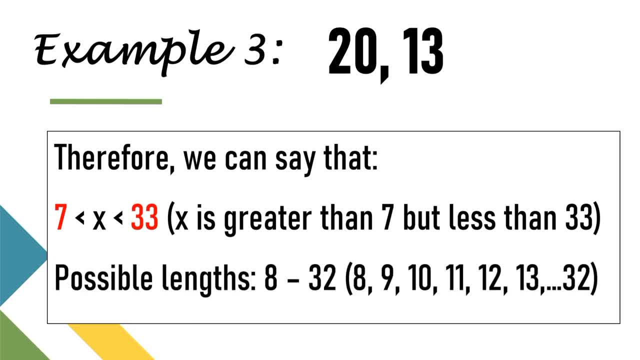 say that x is greater than 7 but less. say that x is greater than 7 but less than 33. so we have here our possible than 33. so we have here our possible than 33. so we have here our possible length: 8 to 32. so the numbers that uh. 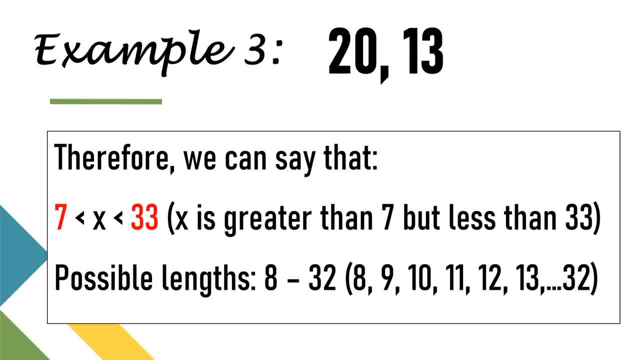 length 8 to 32. so the numbers that uh length 8 to 32. so the numbers that uh starting from 8 and last by 32. so we starting from 8 and last by 32, so we starting from 8 and last by 32. so we have here 8, 9, 10, 11, 12, 13 and up to 32. have here 8, 9, 10, 11, 12, 13 and up to 32. have here 8, 9, 10, 11, 12, 13 and up to 32. so hindi ko nalang nilagay it's because. so hindi ko nalang nilagay it's because. 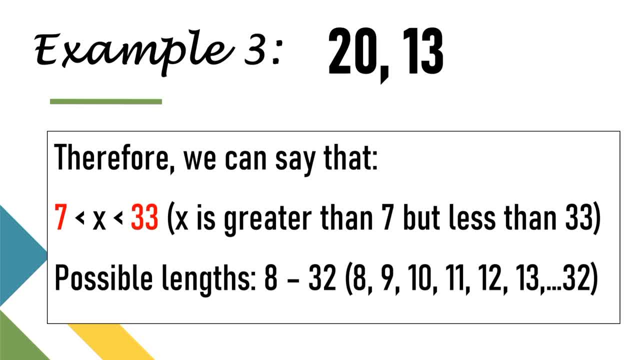 so hindi ko nalang nilagay, it's because masyadong mahaba. so again, when we are masyadong mahaba, so again when we are masyadong mahaba, so again, when we are talking about possible lengths, we have. talking about possible lengths, we have. 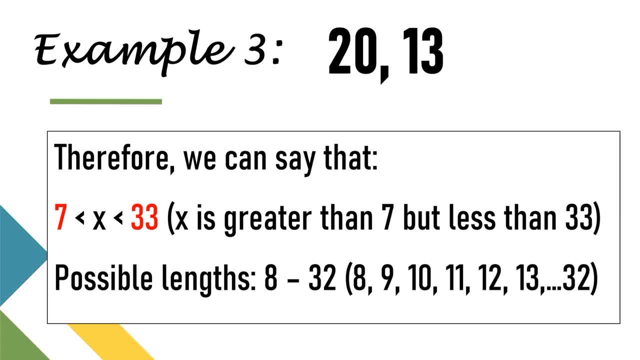 talking about possible lengths. we have here 8 to 32. therefore the number here 8 to 32. therefore the number here 8 to 32, therefore the number starting from 8 up to 32. so 8, 9, 10, 11, 12. 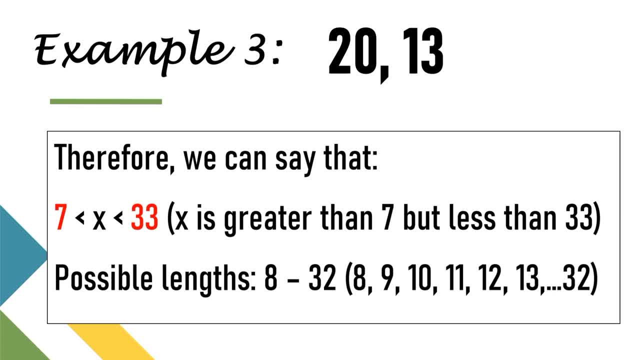 starting from 8 up to 32, so 8, 9, 10, 11, 12. starting from 8 up to 32: so 8, 9, 10, 11, 12, 13, 14, 15 and up to 32, so you can choose. 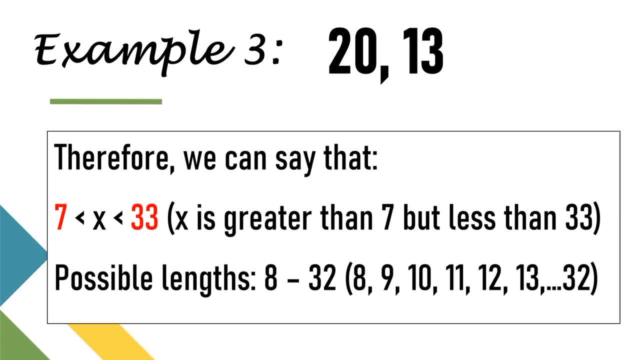 13, 14, 15 and up to 32. so you can choose 13, 14, 15 and up to 32. so you can choose only one to check, okay. so is it clear. only one to check, okay. so is it clear. only one to check, okay. so is it clear, okay, very good. 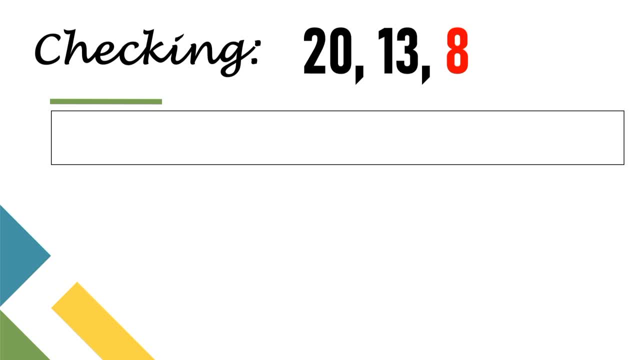 okay, very good, okay, very good, okay, so let's have our checking. we have okay, so let's have our checking. we have okay, so let's have our checking. we have here 20, 13 and 8, okay, so again the here: 20, 13 and 8, okay, so again the. 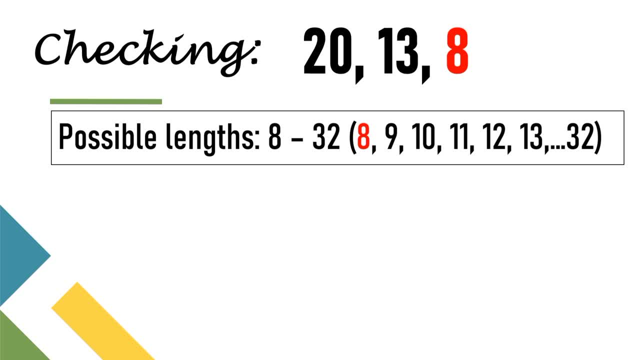 here 20, 13 and 8. okay, so again the possible lengths: we have here 8 to 32 possible lengths. we have here 8 to 32 possible lengths. we have here 8 to 32. we have here 8, 9, 10, 11, 12, 13, 14 and up. 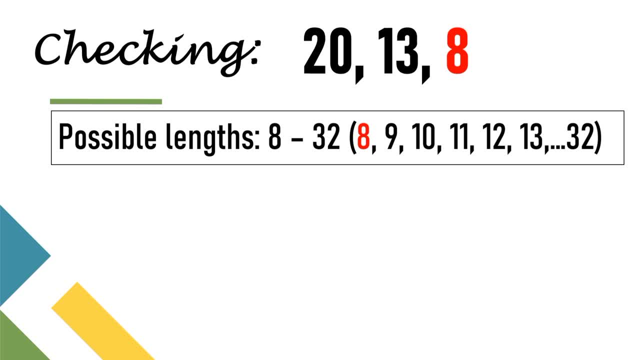 we have here 8, 9, 10, 11, 12, 13, 14 and up. we have here 8, 9, 10, 11, 12, 13, 14 and up to 2 to 2 to 2, uh, 32, okay. so, uh, we have here. 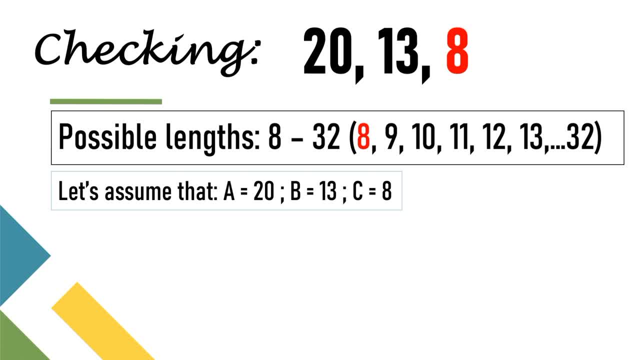 uh 32, okay. so, uh, we have here. uh 32, okay. so, uh, we have here. let's assume that a is equal to 20, b is. let's assume that a is equal to 20, b is. let's assume that a is equal to 20, b is equal to 13 and c is equal to 18. okay, 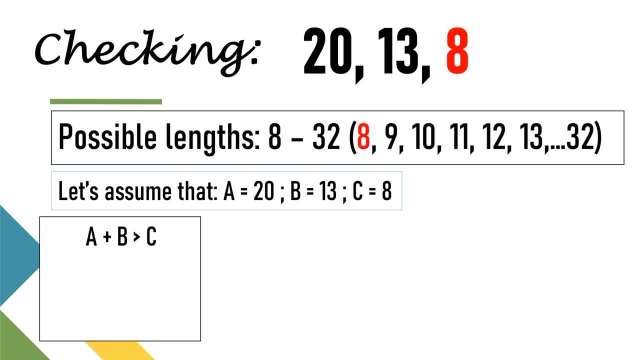 equal to 13 and c is equal to 18. okay, equal to 13 and c is equal to 18. okay, so let's start with the first statement. so let's start with the first statement. so let's start with the first statement. so we have here: a plus b is greater than. 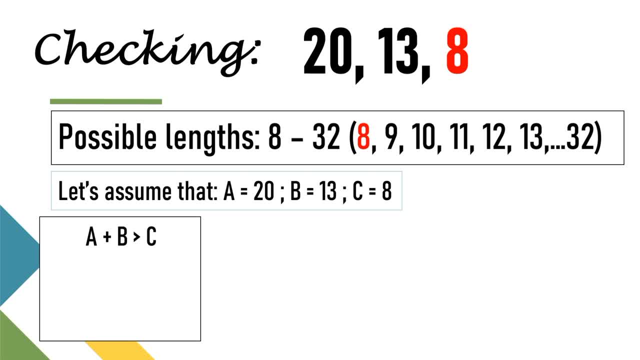 so we have here: a plus b is greater than so. we have here a plus b is greater than c again. all we need to do is to c again. all we need to do is to c again. all we need to do is to substitute the value of our a is 20 and. 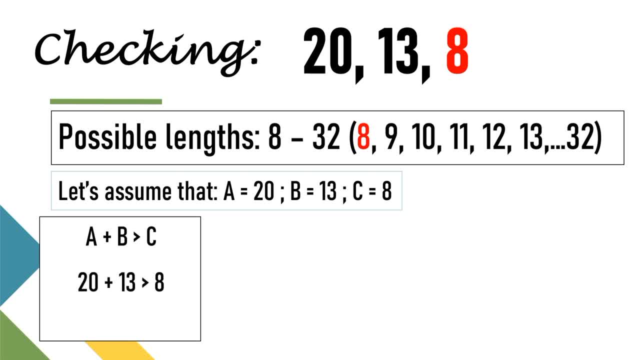 substitute the value of our a is 20 and substitute the value of our a is 20 and the value of our b is 13. we have here: the value of our b is 13. we have here: the value of our b is 13. we have here: 20 plus 13 is greater than the value of. 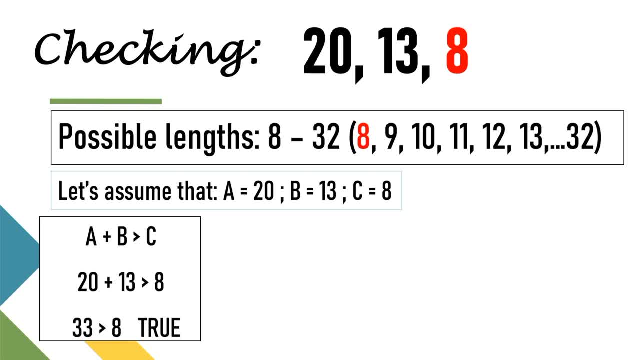 20 plus 13 is greater than the value of our c is 8. so 20 plus 13 we have here. our c is 8. so 20 plus 13 we have here. our c is 8. so 20 plus 13 we have here 33 is greater than 8. and our first: 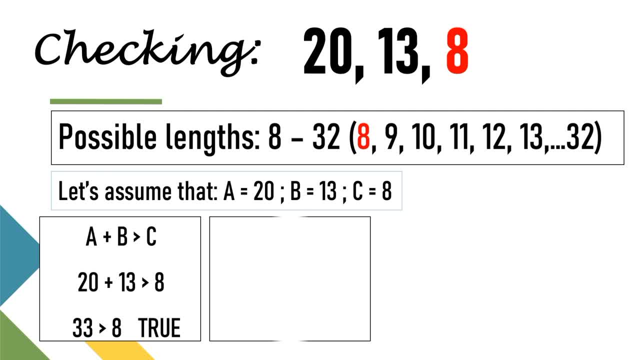 33 is greater than 8 and our first 33 is greater than 8, and our first statement is true: okay, so proceed. is the statement is true? okay, so proceed. is the statement is true? okay, so proceed. is the second statement we have here a plus c. 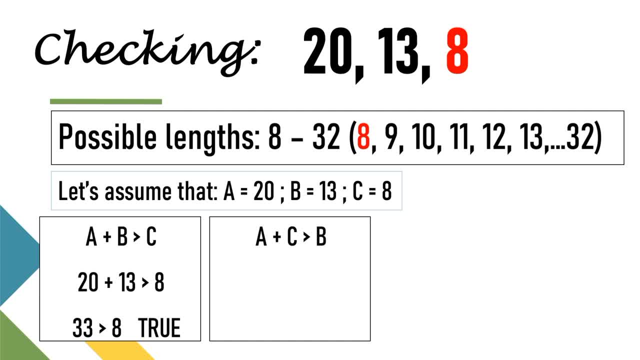 second statement: we have here: a plus c. second statement: we have here: a plus c is greater than b, then the value of our is greater than b, then the value of our is greater than b, then the value of our a is equal to 20 and the value of our c is. 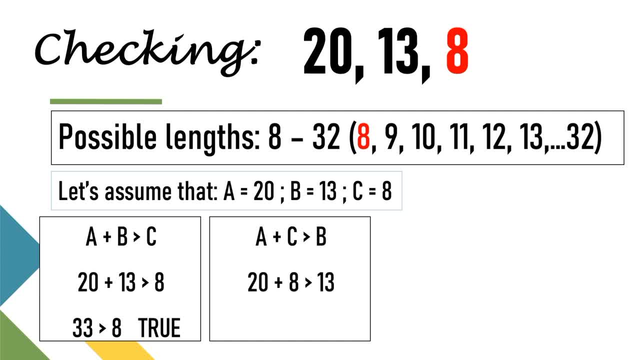 a is equal to 20 and the value of our c is: a is equal to 20 and the value of our c is equal to 8. so 20 plus 8 is greater, equal to 20 and the value of our c is greater than the value of our b is equal. 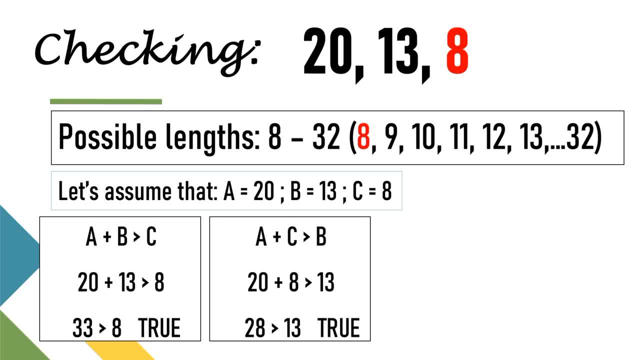 than the value of our b is equal than the value of our b is equal to 13. so 20 plus 8- we have here 28- is to 13. so 20 plus 8- we have here 28- is to 13. so 20 plus 8- we have here 28- is greater than 13. and our second: 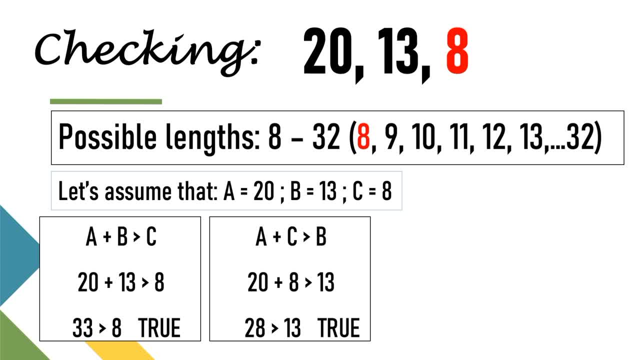 greater than 13 and our second greater than 13. and our second statement is: statement is statement is true, okay, so proceed. is the third: true, okay, so proceed. is the third: true, okay, so proceed. is the third statement. we have here our third statement. we have here our third. 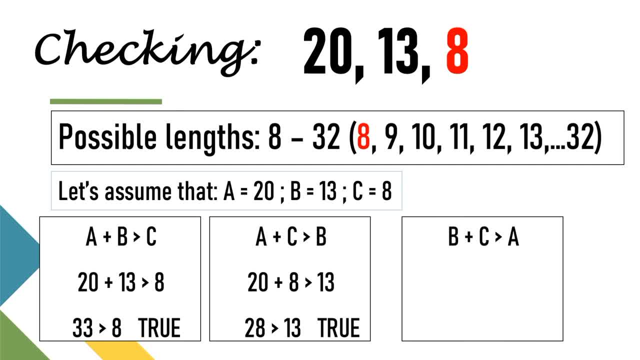 statement. we have here our third statement: b plus c is greater than a. statement b plus c is greater than a. statement b plus c is greater than a. okay, so again, all we need to do is to okay. so, again, all we need to do is to. okay. so again, all we need to do is to substitute: the value of our b is equal. 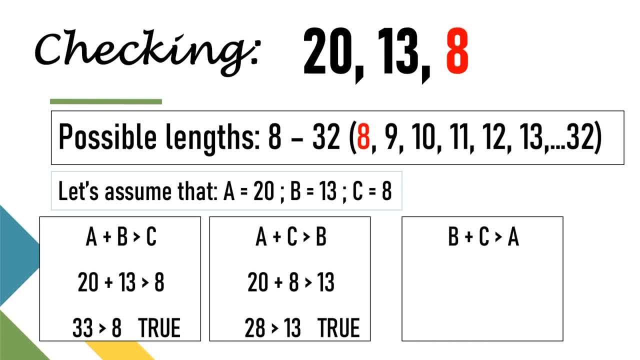 substitute: the value of our b is equal. substitute: the value of our b is equal to 13 and the value of our c is equal to to 13 and the value of our c is equal to to 13 and the value of our c is equal to 8 is greater than. 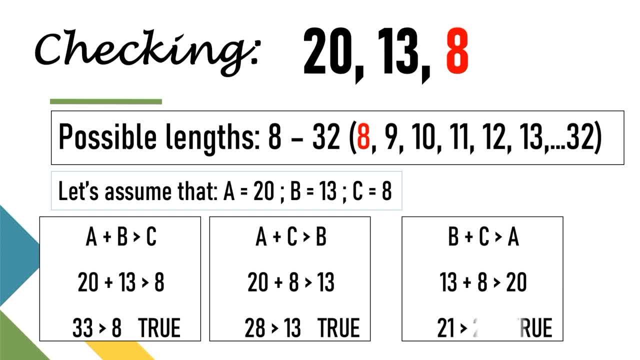 8 is greater than. 8 is greater than. the value of our a is equal to 20, so 13. the value of our a is equal to 20, so 13. the value of our a is equal to 20, so 13 plus 8. we have here 21 is greater than. 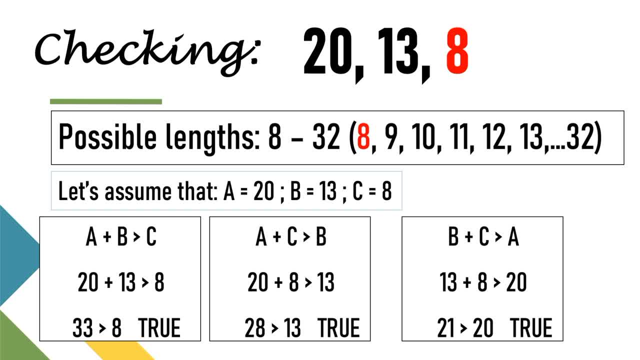 plus 8. we have here 21 is greater than plus 8. we have here 21 is greater than 20. therefore, our third statement is 20. therefore, our third statement is 20. therefore, our third statement is true. okay, so gonna know how to check. 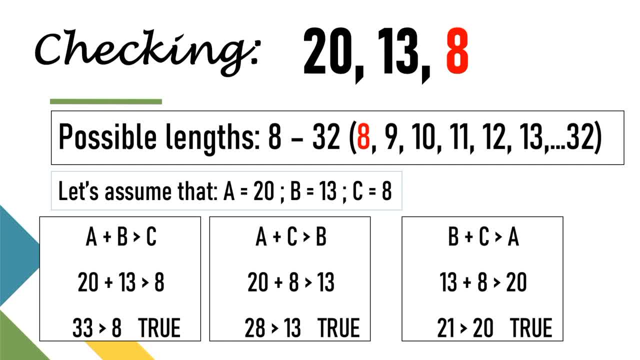 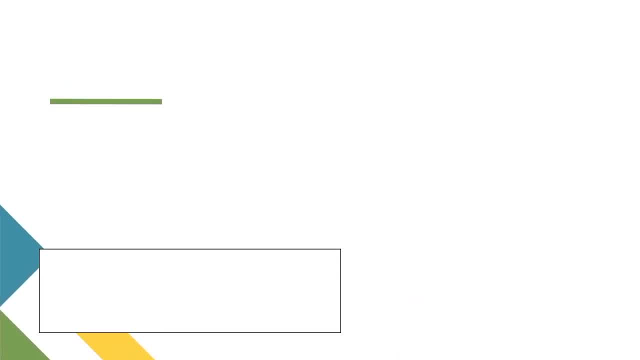 true, okay, so gonna know how to check. true, okay, so gonna know how to check if a possible length, if a possible length, if a possible length, i, okay, so is it clear. okay, very good, okay, so we are done with our third. okay, so we are done with our third. 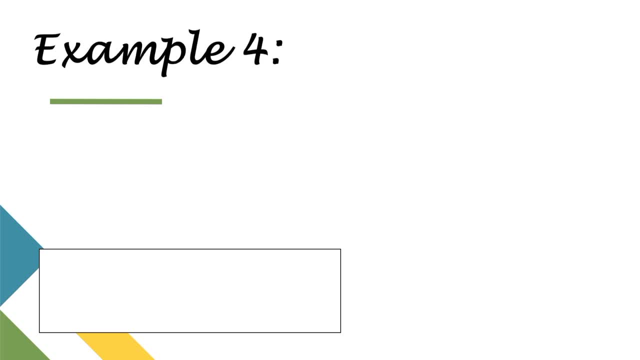 okay, so we are done with our third example. so now example. so now example. so now proceed, for example. or example number, proceed, for example. or example number. proceed, for example. or example number four. so we are given here four. so we are given here four. so we are given here, uh, two sides, the nine and nine. okay, or? uh, two sides- the nine and nine- okay, or uh, two sides- the nine and nine- okay, or the measurement of the two sides. so we the measurement of the two sides, so we the measurement of the two sides. so we have here nine and nine, have here nine and nine. 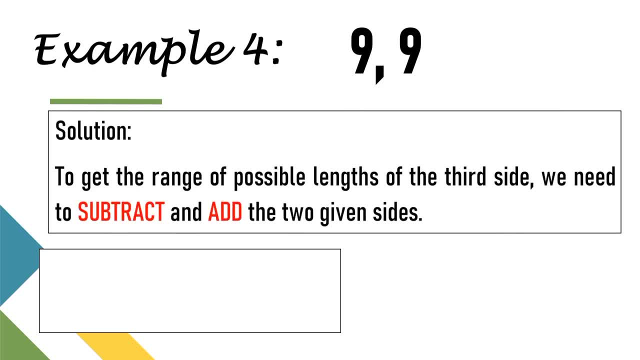 have here nine and nine. so again to get the range of possible. so again to get the range of possible. so again to get the range of possible. lengths of the third side, lengths of the third side, lengths of the third side. we need to subtract and add the two. 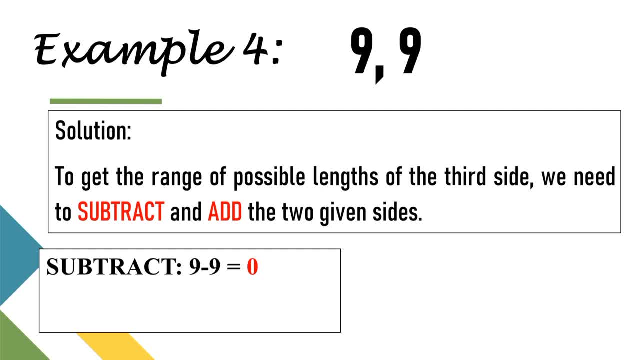 we need to subtract and add the two. we need to subtract and add the two. given sides, so given sides, so given sides. so let's start with subtraction. so we have, let's start with subtraction. so we have, let's start with subtraction. so we have here: subtract nine by nine, so nine minus. 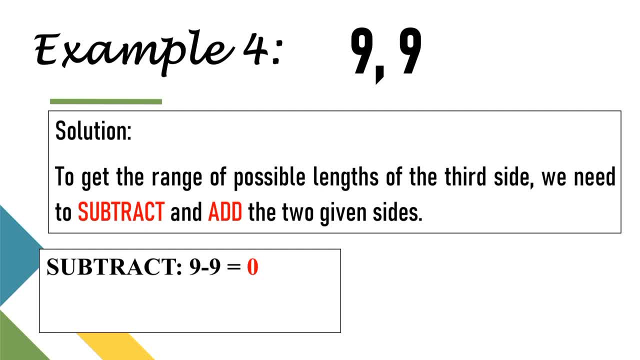 here. subtract nine by nine, so nine minus here. subtract nine by nine, so nine minus nine. we have here nine. we have here nine. we have here zero. so we are done with our subtraction zero. so we are done with our subtraction zero. so we are done with our subtraction. proceed to addition. so we have here: 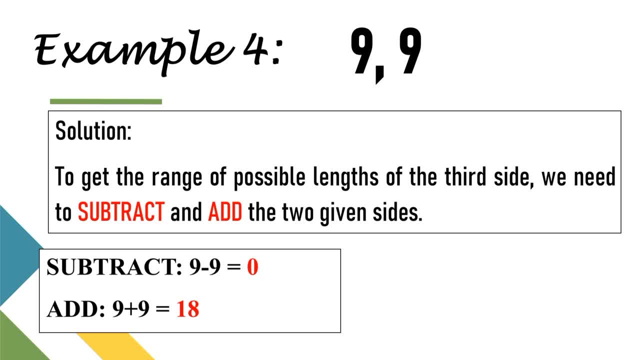 proceed to addition. so we have here: proceed to addition. so we have here our addition nine plus nine. so the result: our addition nine plus nine. so the result: our addition nine plus nine. so the result: or the sum is equal to, or the sum is equal to, or the sum is equal to 18, so again the difference is zero, and 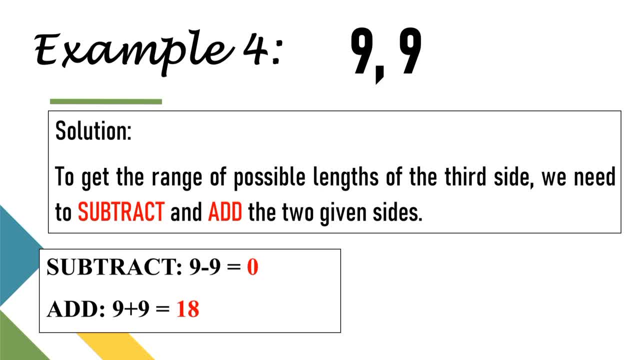 18. so again the difference is zero and 18. so again the difference is zero and the sum is 18. or let me say the sum is 18, or let me say the sum is 18, or let me say the result of the subtraction we have. 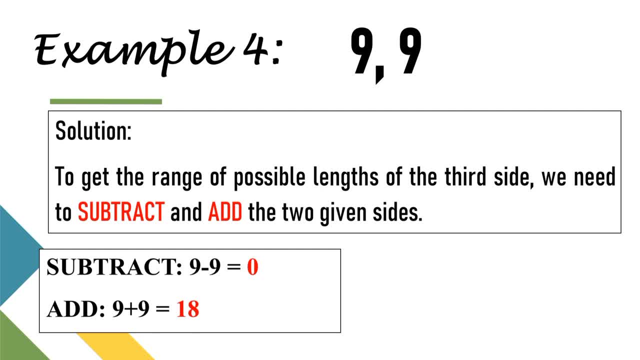 the result of the subtraction we have, the result of the subtraction we have: here zero, here zero, here zero, and the result of our addition is equal, and the result of our addition is equal and the result of our addition is equal to 18, 18, so to 18, 18 so. 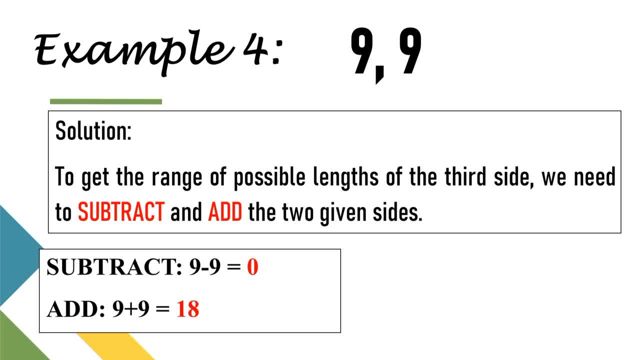 to 18. 18, so uh don't forget with that one, okay, zero, uh don't forget with that one, okay, zero, uh don't forget with that one, okay, zero. and 18: okay, so is it here. and 18. okay, so is it here. and 18. okay, so is it here? okay, very good. 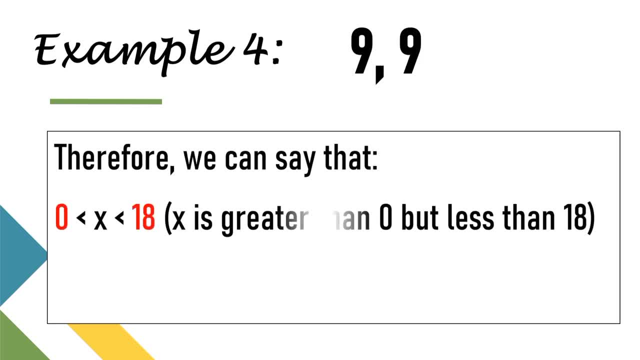 okay. so we have here. therefore, we can say okay, we can say okay, we can say that x is greater than zero, but less than that x is greater than zero, but less than that x is greater than zero, but less than 18. so again, 18, so again. 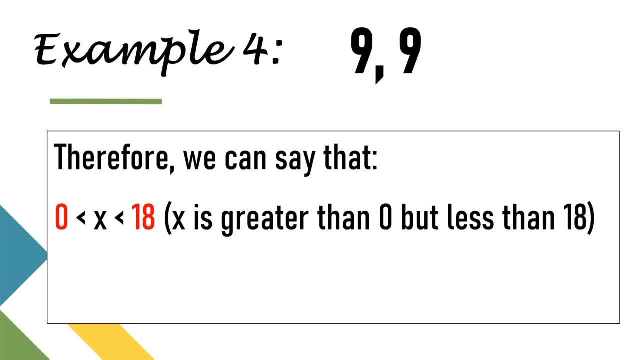 18. so, again, the result of the subtraction, which is the result of the subtraction, which is the result of the subtraction which is zero, then zero, then zero, then greater than sine, then x, then less than greater than sine, then x, then less than greater than sine, then x, then less than sine, and the result of the addition. so, 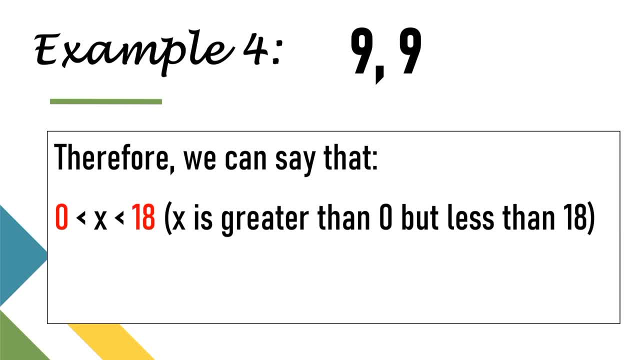 sine and the result of the addition. so sine and the result of the addition. so that's why this, that's why this, that's why this: it says that x is greater than zero, but it says that x is greater than zero, but it says that x is greater than zero but less than 18.. so the possible lengths: 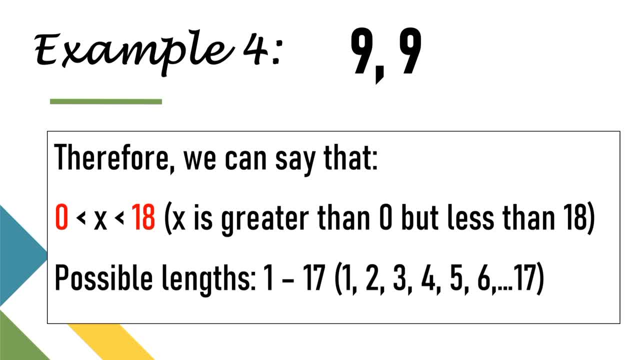 less than 18.. so the possible lengths: less than 18.. so the possible lengths here we have, uh, the number that is here. we have, uh, the number that is here. we have, uh, the number that is greater than zero. we have here one greater than zero. we have here one. 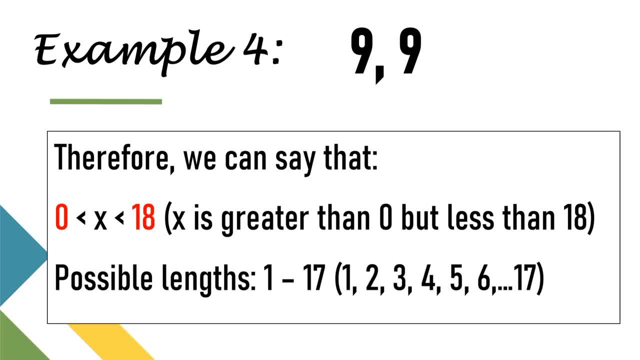 greater than zero. we have here one minus minus minus, or 1 to 17, rather so 1 to 17, so we can. or 1 to 17, rather so 1 to 17, so we can. or 1 to 17, rather so 1 to 17, so we can say that the possible length is we have. 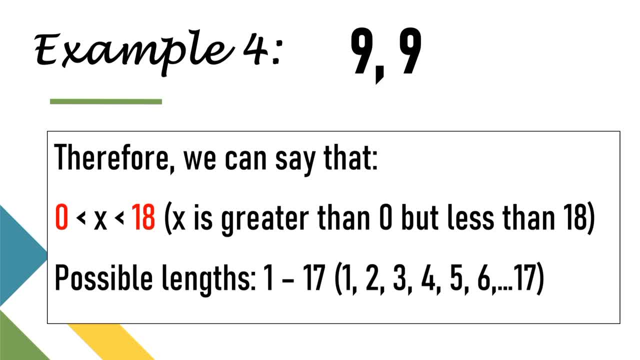 say that the possible length is. we have say that the possible length is. we have a 1, 2, 3, 4, 5, 6, up to 17.. so again, a 1, 2, 3, 4, 5, 6, up to 17.. so again, 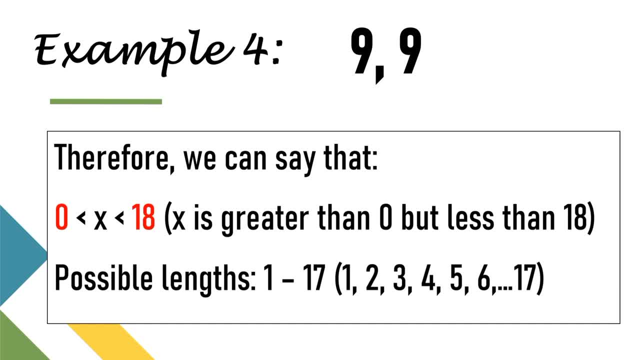 a: 1, 2, 3, 4, 5, 6, up to 17.. so again, hindi ko nilagay, it's because hindi ko nilagay, it's because hindi ko nilagay, it's because masyadong mahaba. so it's up to you. if 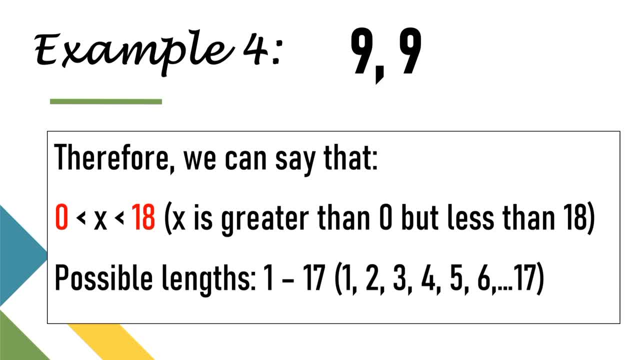 masyadong mahaba, so it's up to you. if masyadong mahaba, so it's up to you. if you will uh pick uh one number, okay, you will uh pick uh one number. okay, you will uh pick uh one number. okay, para mag check. okay, so again, para mas. 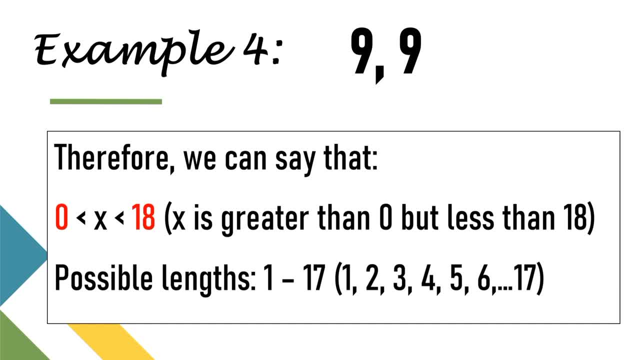 para mag check. okay. so again para mas para mag check. okay. so again para mas. madali sa inyo, you can choose only one. madali sa inyo, you can choose only one. madali sa inyo, you can choose only one para sa checking. okay, so is it clear. 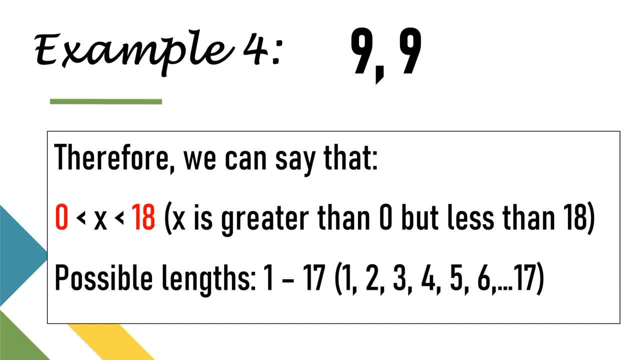 para sa checking okay, so is it clear. para sa checking okay, so is it clear, okay, very good. so again x greater than okay, very good, so again x greater than okay, very good. so again x greater than zero, but less than 18, so therefore our zero, but less than 18, so therefore our. 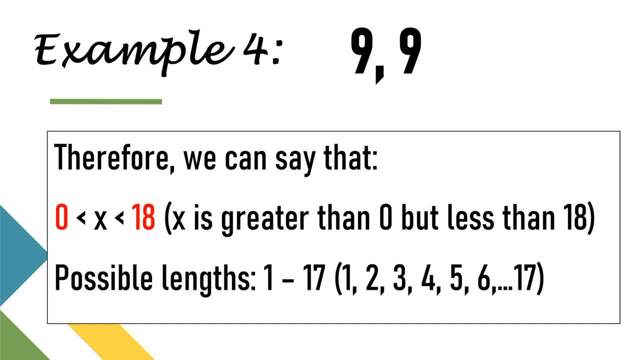 zero but less than 18. so therefore our possible lines: we have here 1, 2, 17, so possible lines: we have here 1, 2, 17, so possible lines: we have here 1, 2, 17. so we have here 1, 2, 3, 4, 5, 6 up to 17. we have here 1, 2, 3, 4, 5, 6 up to 17. we have here: 1, 2, 3, 4, 5, 6 up to 17. the numbers okay, so is it clear, okay, very. the numbers okay, so is it clear, okay, very. 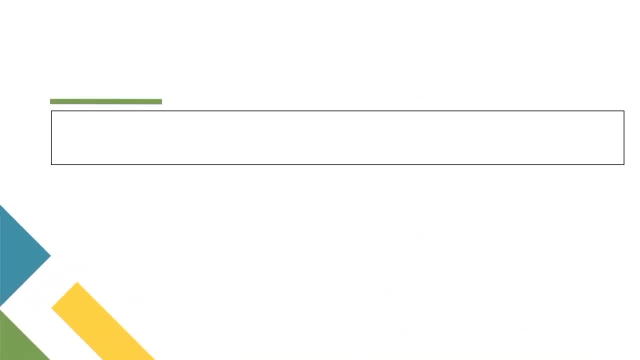 the numbers. okay, so is it clear? okay, very good, good, good, okay, so we have here our checking. we okay, so we have here our checking. we okay, so we have here our checking. we have here nine, nine, and have here nine, nine, and have here nine, nine and one. okay, so again the possible lengths. we 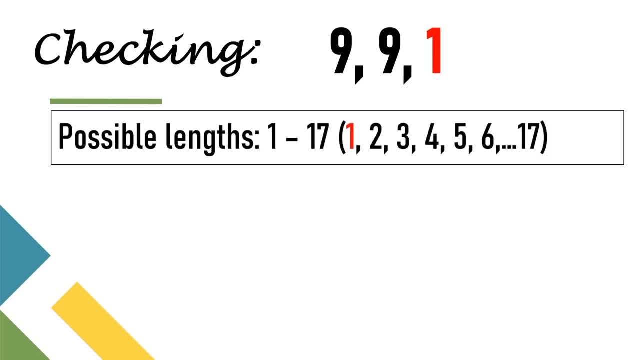 one, okay. so again the possible lengths. we one okay, so again the possible lengths. we have here one, two, seventeen one, two. have here one, two, seventeen one, two. have here one, two, seventeen one. two. three, four, five, six up to 17, so i only three, four, five, six up to 17, so i only. 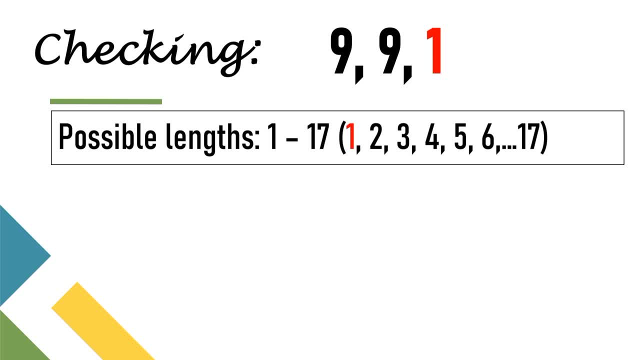 three, four, five, six, up to 17. so i only choose one number. para choose one number. para choose one number. para mag serve as the third side. so let's mag serve as the third side. so let's mag serve as the third side. so let's assume that a is equal to nine, b is 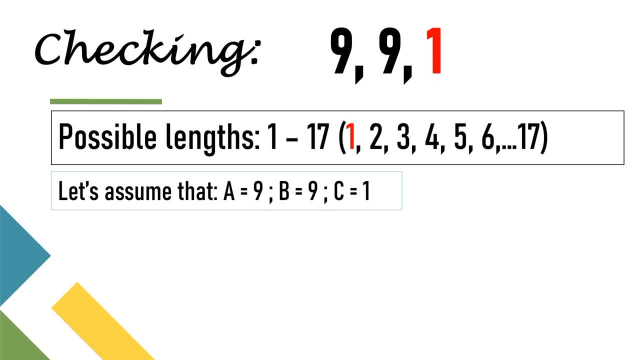 assume that a is equal to nine, b is assume that a is equal to nine, b is equal to nine and c is equal to one, so equal to nine and c is equal to one, so equal to nine and c is equal to one. so let's use, uh, the three statements, okay. 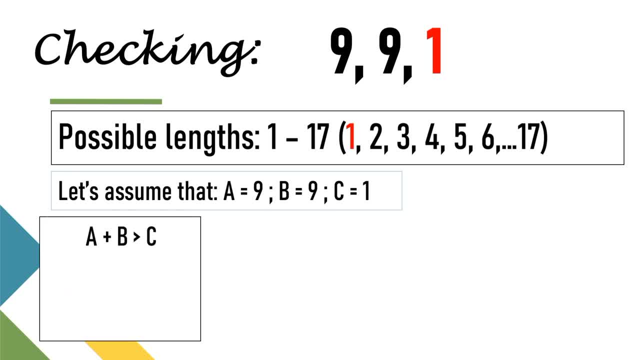 let's use, uh, the three statements, okay. let's use, uh, the three statements okay. so let's check first. so let's check first. so let's check first. first statement we have here: a plus b is first statement we have here: a plus b is first statement we have here: a plus b is greater than the value of our c is. 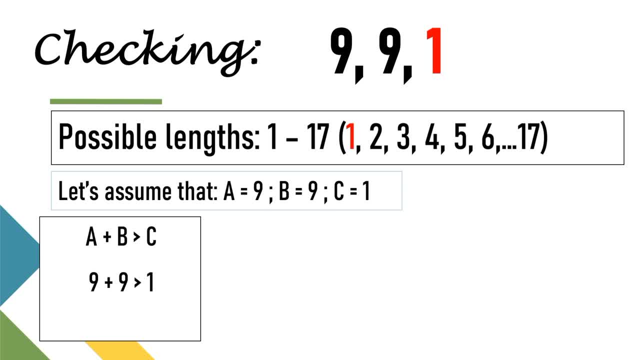 greater than the value of our c is greater than the value of our c is equal to one. so nine plus nine is equal to one. so nine plus nine is equal to one. so nine plus nine is greater than one. so nine plus nine, we greater than one. so nine plus nine, we. 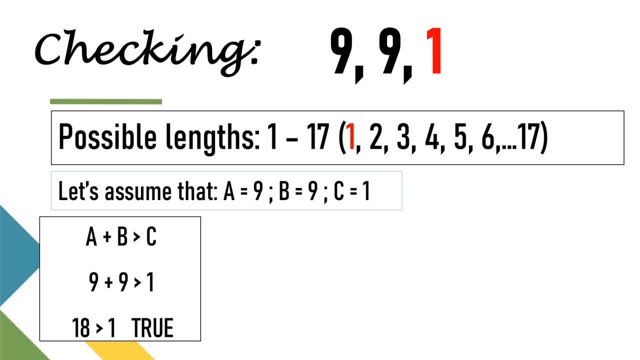 greater than one. so nine plus nine. we have here 18 is greater than one. so our have here: 18 is greater than one. so our have here 18 is greater than one. so our first statement is true: okay, so 19. first statement is true, okay, so 19. 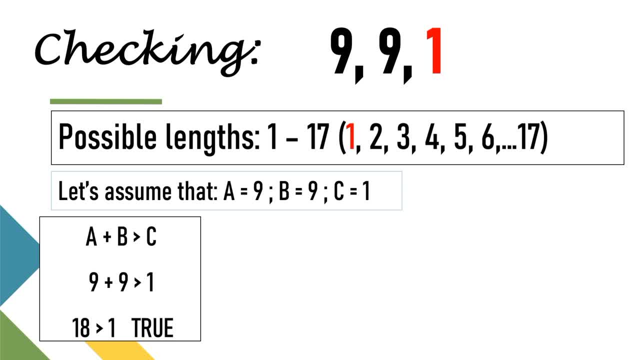 first statement is true, okay, so 19 behind. okay, very good, so let's check behind. okay, very good, so let's check behind. okay, very good, so let's check the second statement. okay, we have here the second statement. okay, we have here the second statement. okay, we have here our second statement, a plus c. 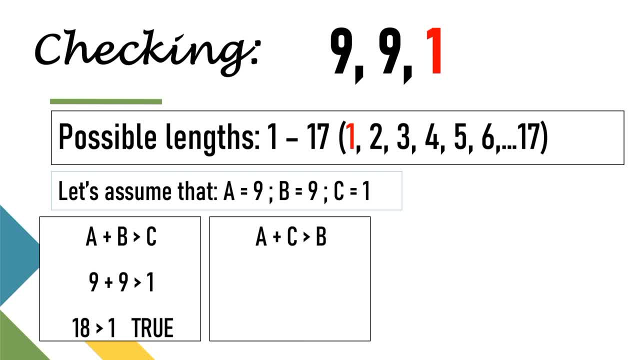 our second statement: a plus c. our second statement: a plus c is greater than b. okay, next one again is greater than b. okay, next one again is greater than b. okay, next one again. all you need to do is to substitute the. all you need to do is to substitute the. 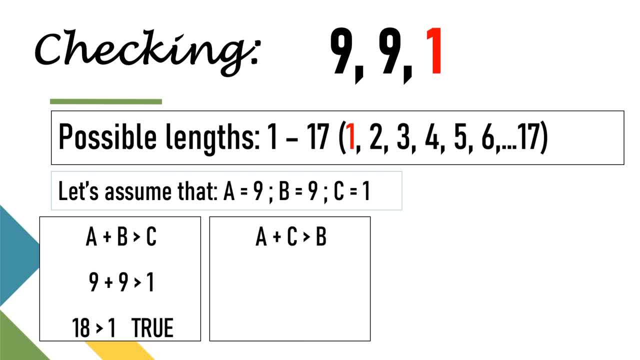 all you need to do is to substitute: the value of our a is equal to nine and the value of our a is equal to nine. and the value of our a is equal to nine and the value of our c is equal to one, so we value of our c is equal to one, so we. 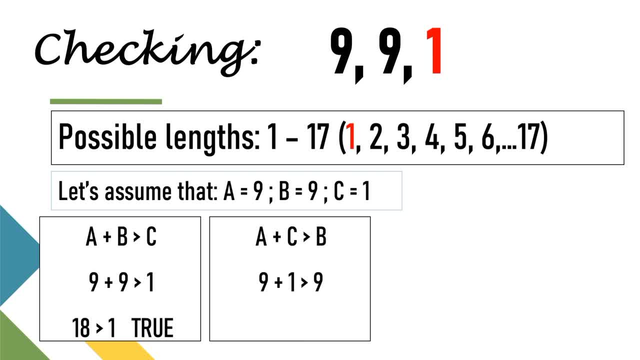 value of our c is equal to one. so we have here: nine plus one is greater than have here. nine plus one is greater than have here. nine plus one is greater than nine. so the value of our b is equal to nine. so the value of our b is equal to. 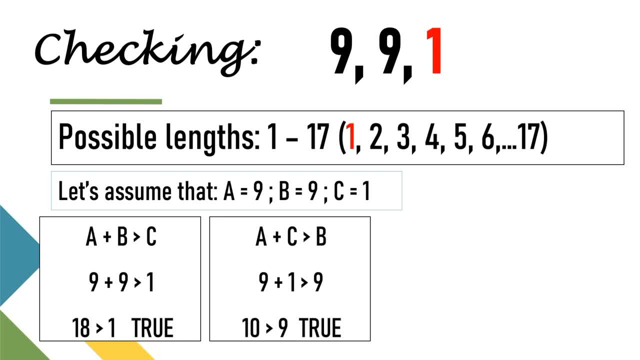 nine. so the value of our b is equal to nine. so nine plus one. we have here ten nine, so nine plus one. we have here ten, nine, so nine plus one. we have here ten is greater than nine. okay, and our first is greater than nine. okay, and our first. 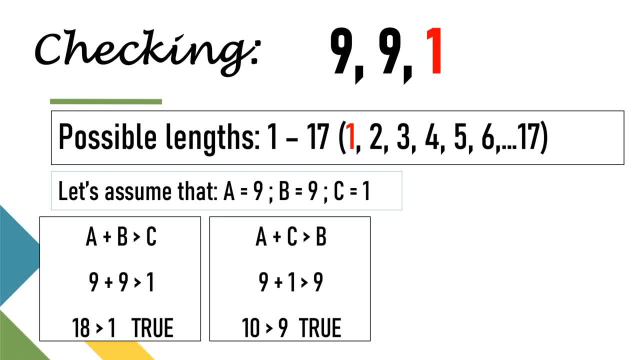 is greater than nine. okay, and our first. our second statement rather is true, okay. our second statement, rather is true, okay. our second statement, rather is true, okay. so 19 behind, okay, very good. so again. so 19 behind, okay, very good. so again. so 19 behind, okay, very good. so again, ten is greater than nine. therefore, our 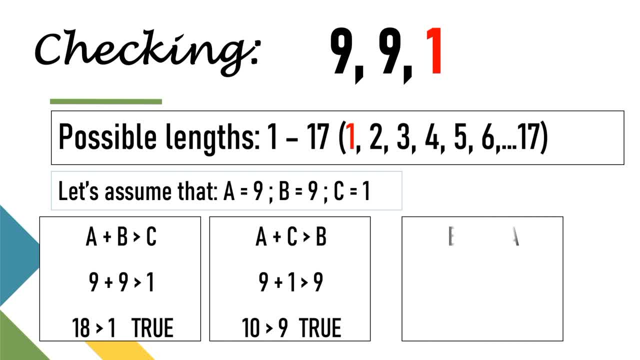 ten is greater than nine. therefore, our ten is greater than nine. therefore, our second statement is true: okay, so proceed. second statement is true: okay, so proceed. second statement is true: okay, so proceed. is the third statement, so we have here. is the third statement, so we have here. 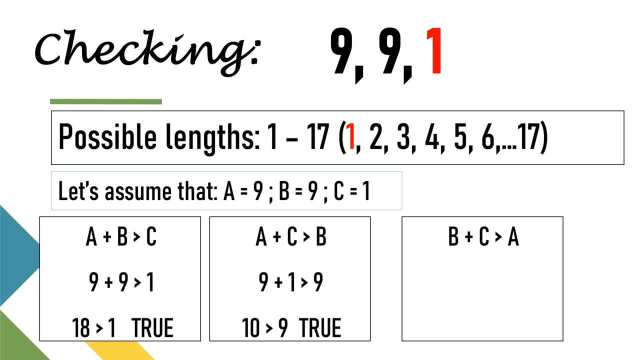 is the third statement. so we have here our third statement: b plus c is greater. our third statement: b plus c is greater. our third statement: b plus c is greater than a. so the value of our b is equal than a. so the value of our b is equal. 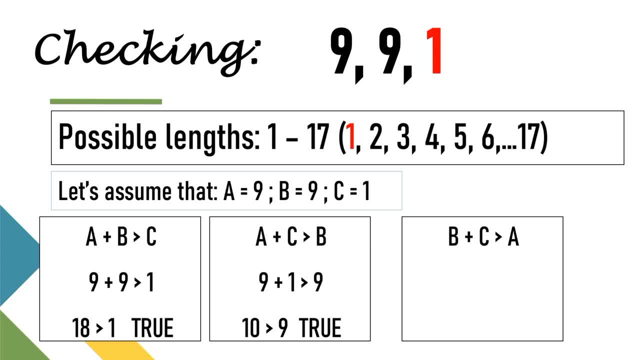 than a. so the value of our b is equal to nine plus the value of our c is equal to nine plus the value of our c is equal to nine plus the value of our c is equal to one. so nine plus one is greater than to one. so nine plus one is greater than. 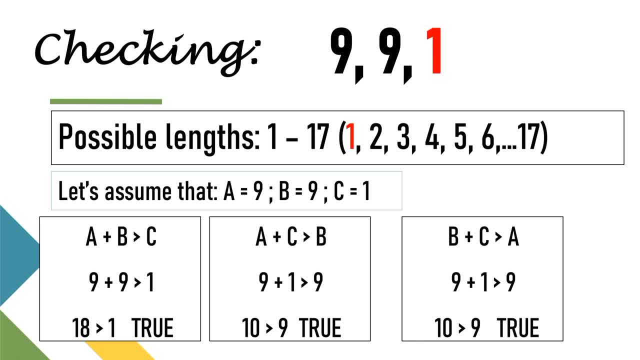 to one. so nine plus one is greater than nine. so nine plus one. we have here ten nine. so nine plus one, we have here ten nine. so nine plus one- we have here ten- is greater than the value of our a is is greater than the value of our a is. 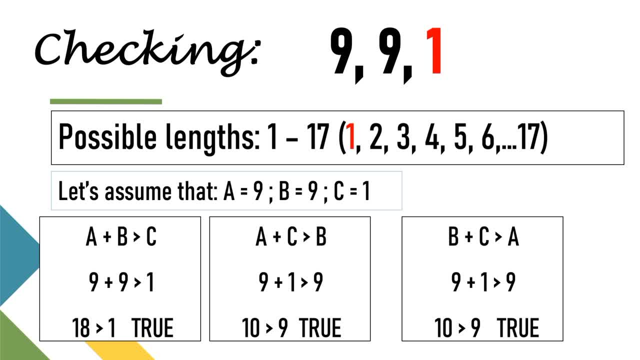 is greater than the value of our a is equal to, equal to equal to nine, so ten is greater than nine, nine, so ten is greater than nine, nine, so ten is greater than nine. therefore, our third statement is: therefore: our third statement is, therefore, our third statement is true. so therefore, class, we can say that. 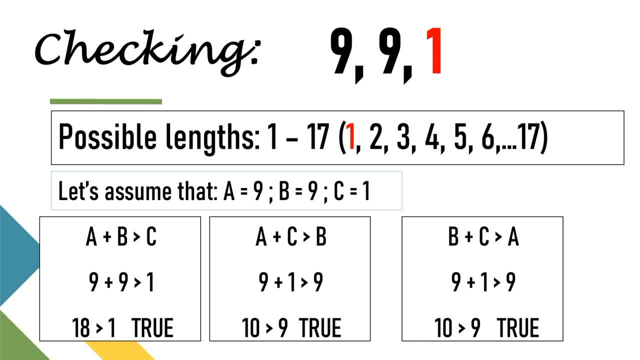 true. so therefore, class, we can say that true. so therefore, class, we can say that the possible length can represent the. the possible length can represent the. the possible length can represent the length of the third side of the given length, of the third side of the given length, of the third side of the given triangle. okay, so 90 hand, 90 hand back.